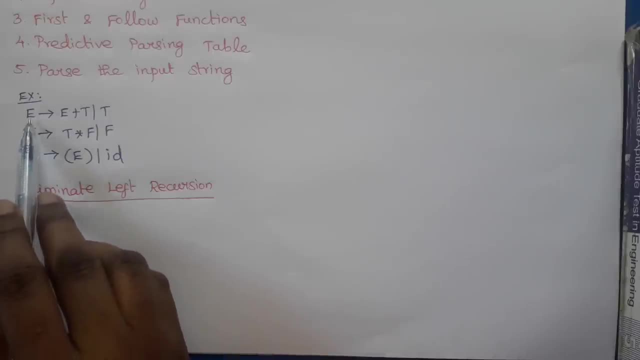 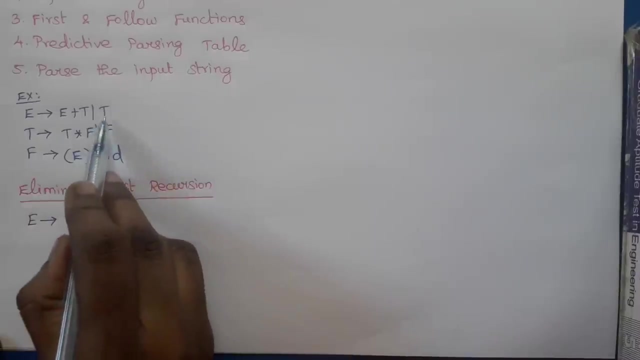 grammar. So to eliminate left recursion from the grammar first we need to write the symbol on the left side. so e tends to first write the non-left recursive production, so t all the non-left recursive production for e should be written with the new non-terminal at the end. So here only one. 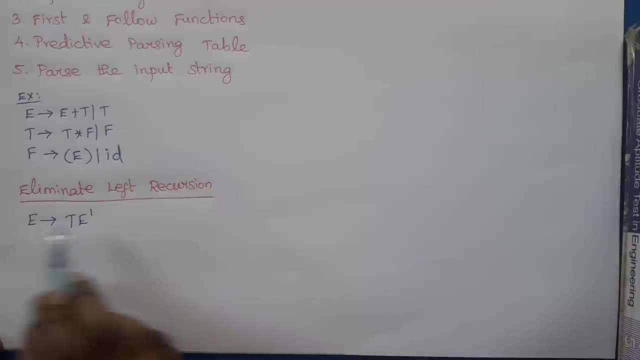 non-left recursive production. so we need to write t, then a new symbol, e dash, new non-terminal. then this new non-terminal symbol e dash gives from the left recursive productions. write all symbols except the first one. so plus t, then rewrite the same e dash at the end. 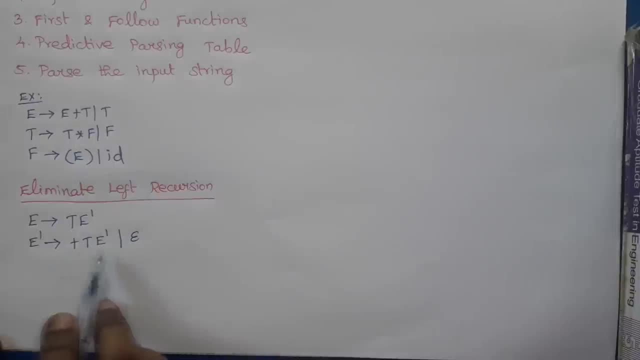 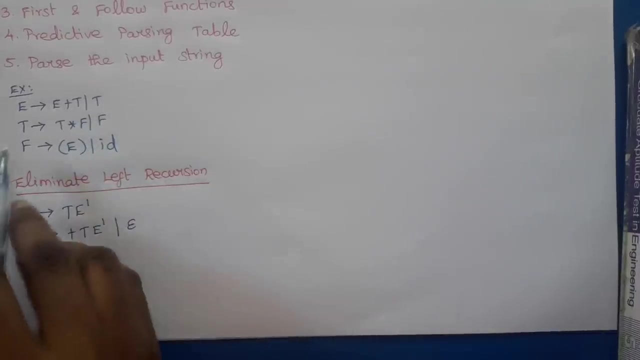 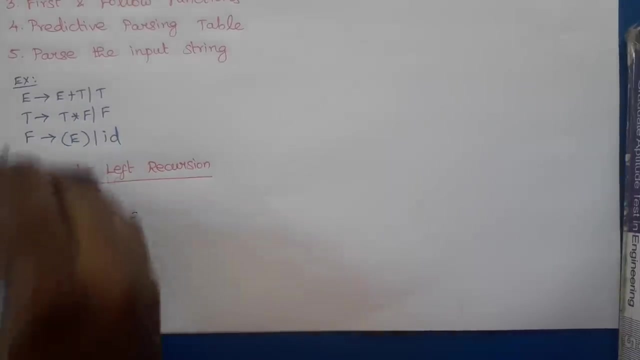 r epsilon. So this is the way to eliminate left recursion. t e dash, then e dash tends to plus e dash, T E dash bar epsilon. So T is also having left recursive, left recursion. So we need to eliminate from T. So T gives non-left recursive production is F, then introduce a non new, non-terminal. 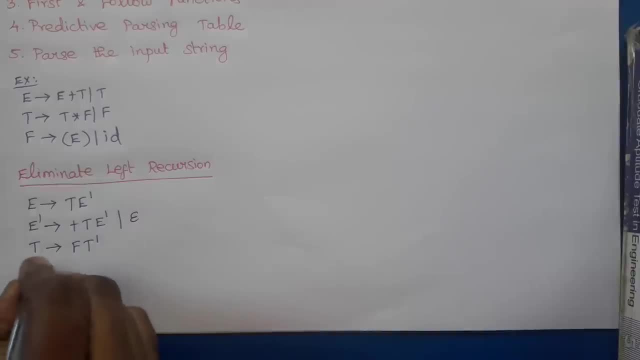 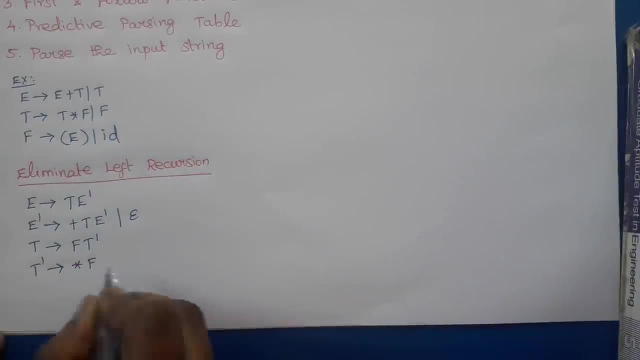 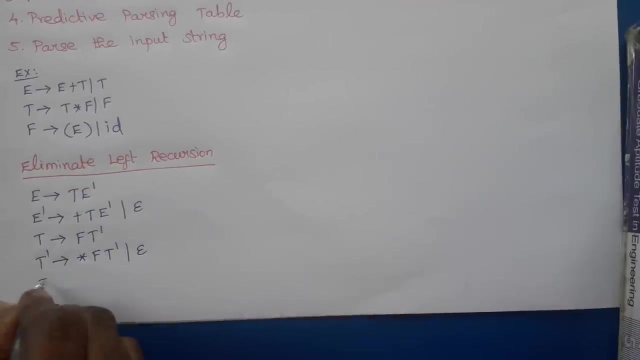 corresponding to T, So T dash. then this T dash gives star F. write all symbols except the first, So star F. then rewrite the new symbol, T dash, bar epsilon. Since F is not a left recursive production, do not eliminate anything or do not rewrite it, just write the same production. 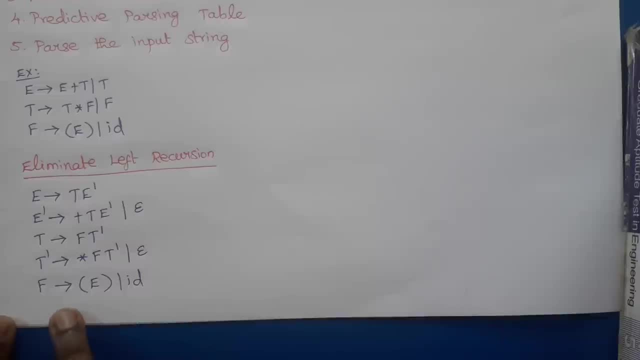 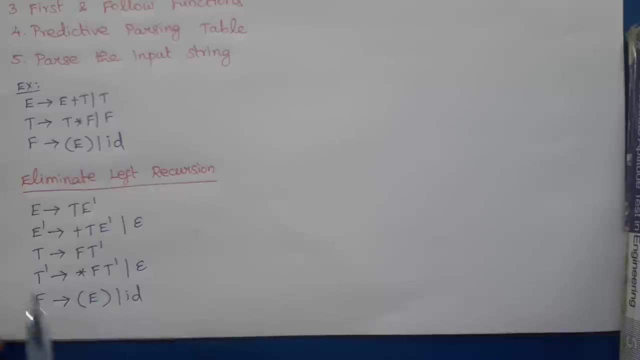 So here we have eliminated left recursion from the grammar. Next we need to check left factoring is possible or not. So this is a resulting grammar after eliminating left recursion. So here we need to check left factoring is possible. So left is possible or not. that is, the productions are having common symbols from the left end. 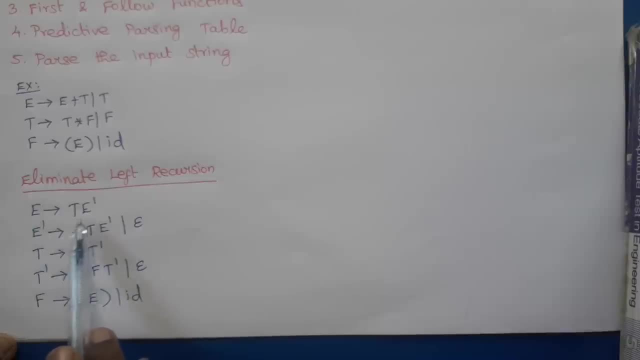 This production is having only one, only one production. E has only one production, right, so no need to check anything. here has two productions. E dash as two productions. but first starts with plus. here epsilon. here only one production, the star and epsilon open-end IdSo left factoring is not possible. so third step is we need to do the first and 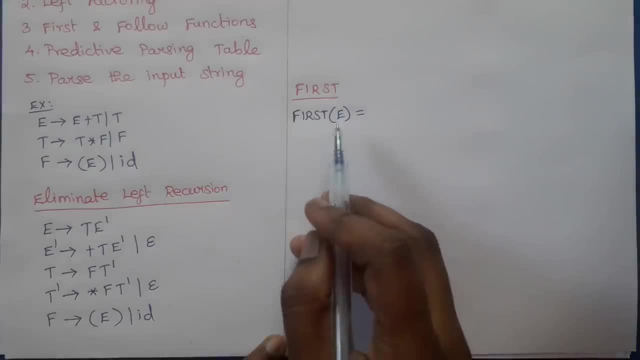 follow function. So first step is a start point, So start point. so it will be a start point. So as a So first we need to find first of the non-terminal E. So there are. in the previous video we have seen 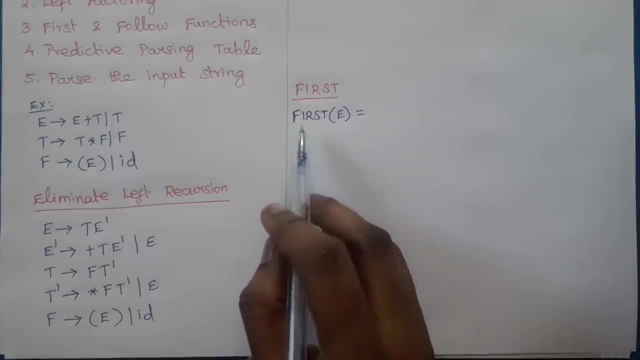 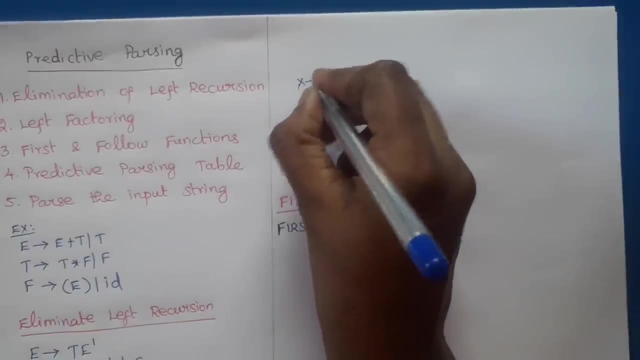 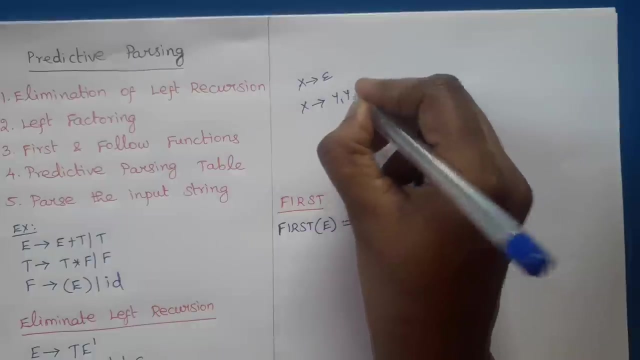 how to find first and follow functions. So first of terminal symbol is terminal symbol. This is first rule. Second rule is: if x tends to epsilon is a production, then first of x is epsilon. Then third rule is: if x tends to y1, y2 up to yk, If this is a production, then first of x is. 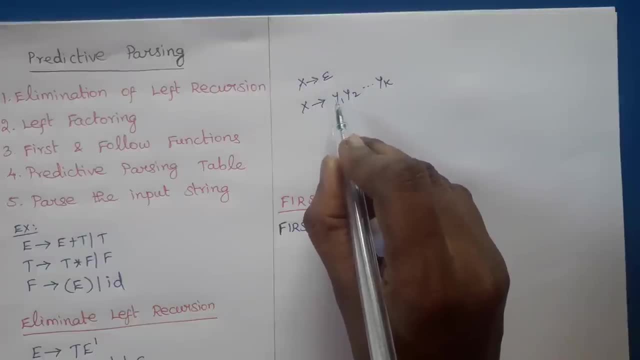 first of y1. That is, we need to include all symbols of first of y1 to first of x, except epsilon. Suppose first of y1 is having epsilon, we need to include all symbols in first of y2 also, If y2 is also having epsilon, then we need to include first of y3. So similarly we have. 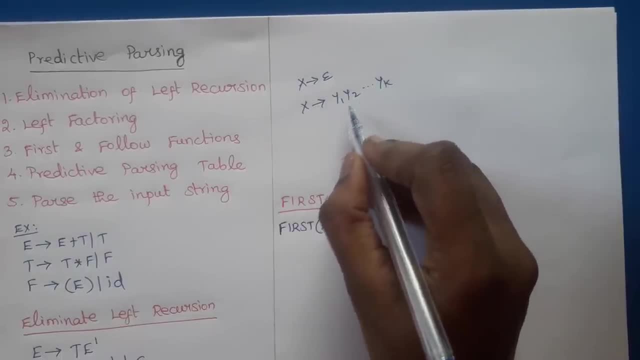 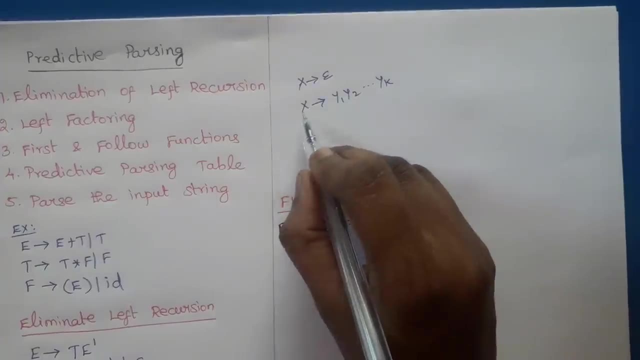 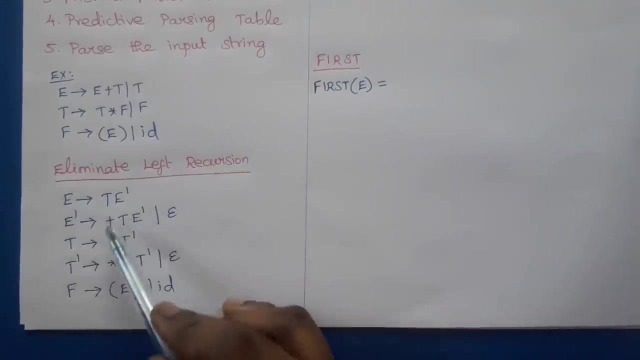 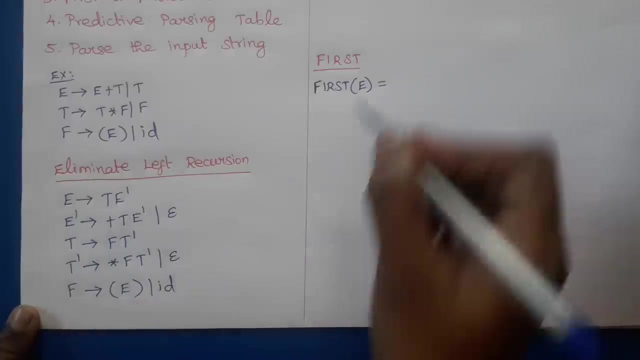 to do this. If all the symbols are having epsilon, first of all the symbols, k symbols are having epsilon, Then we need to add epsilon to x. So this is a rule for finding first. So first of e, First we need to find first of e. First of e means here third rule is applied. So first of e is first of t. 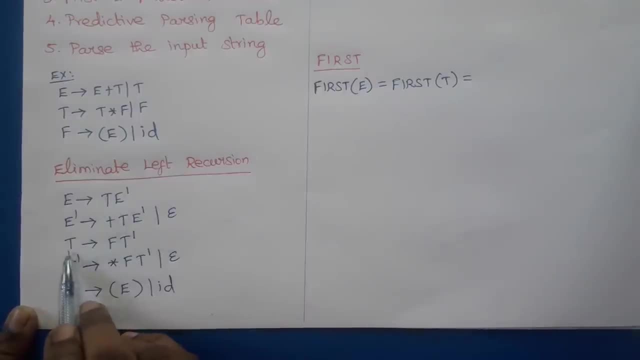 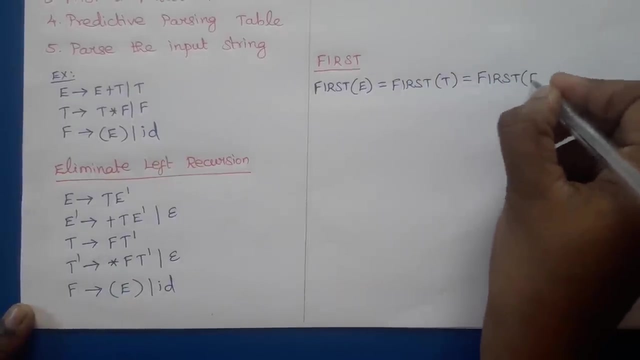 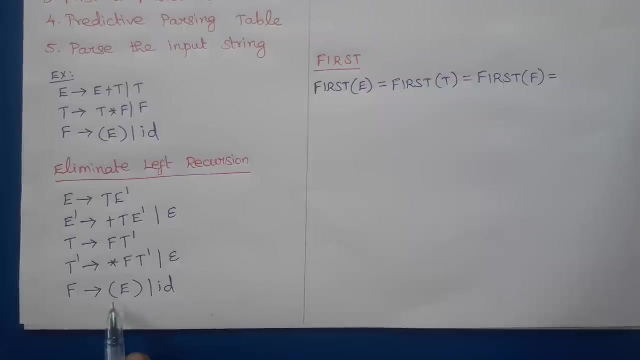 So we need to find first of t, What is first of t, First of f. So first of t is first of f. So we have to find first of f. First of f means we need to consider the two productions. So first production it starts with left parenthesis. So first of the terminal symbol is: 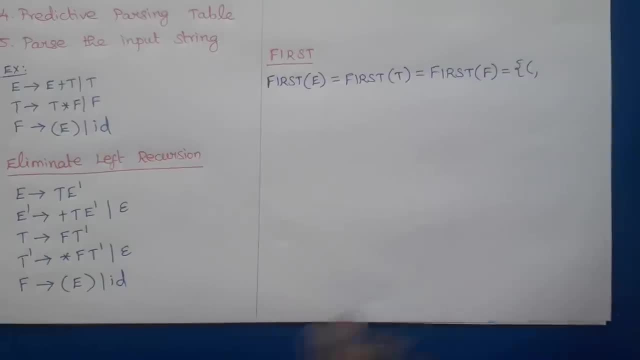 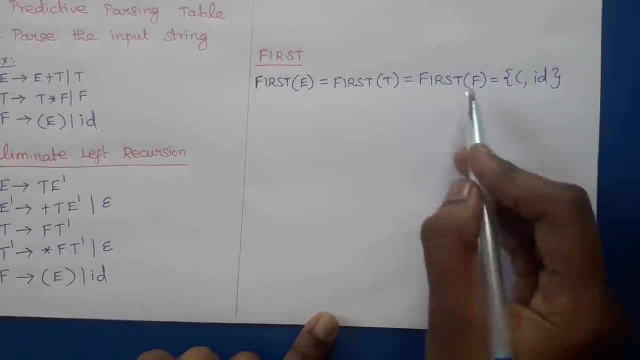 terminal symbol, So left parenthesis. Then if we consider the second production, it, the second production also starts with the terminal symbol. So first of f is id also. So first of e, t and f, all are having the same first function: Left parenthesis and id. Now we need to find: first 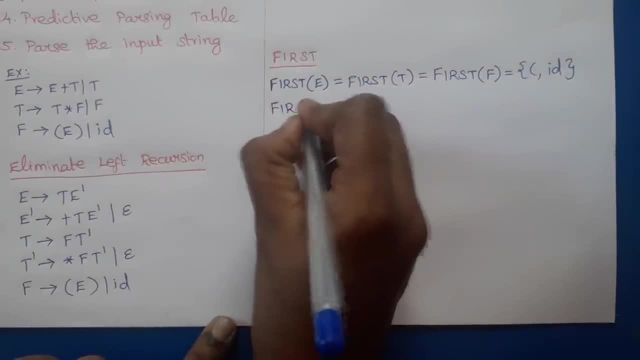 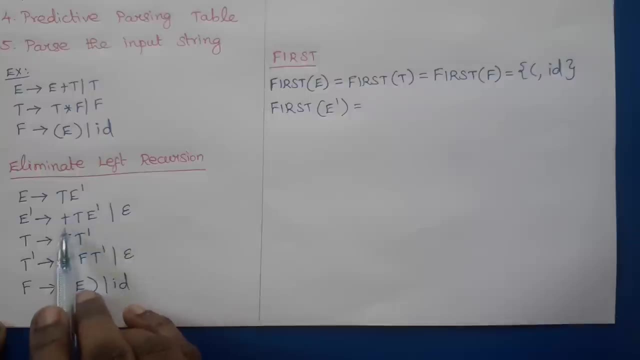 of e dash and t dash. So first of e dash is: first of e dash is: if we consider the first production, it starts with the terminal. So first of plus, First of plus is plus and the second production is e dash tends to epsilon. So if e dash tends to epsilon as a production, first of e dash is 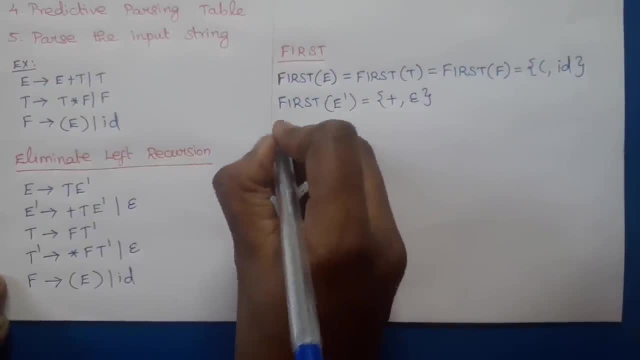 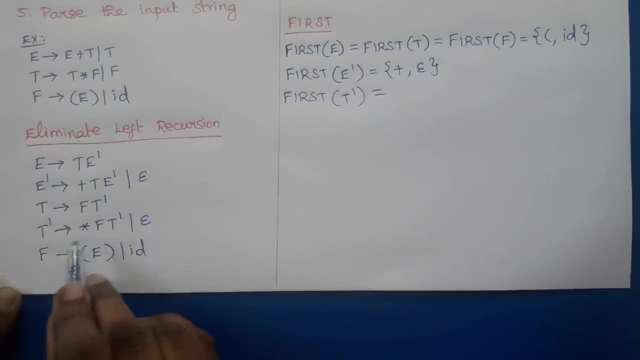 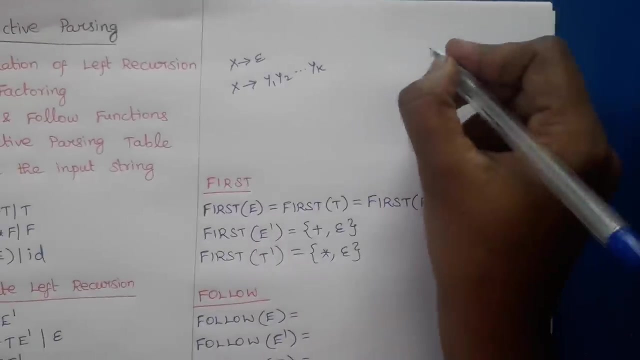 epsilon. Then first of t dash, First of t dash, it starts with terminal symbol. So first of star is star and second production is epsilon, So epsilon. Then we need to find follow for all the non-terminal symbols. So the rule for the follow is first, rule is we need to. 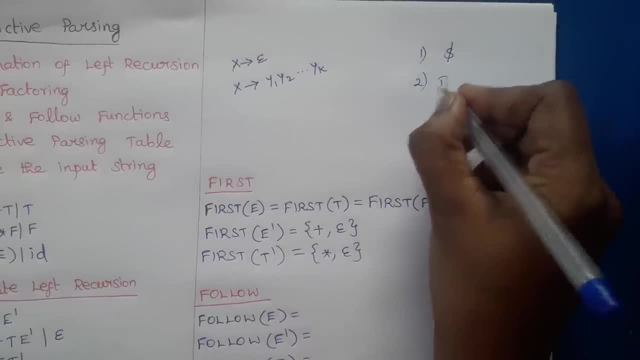 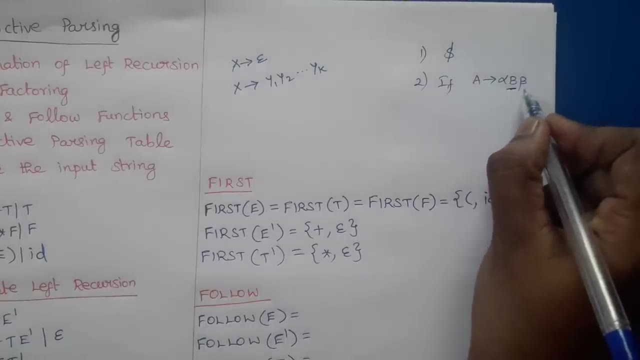 place dollar for the follow of start symbol of the grammar. So if a tends to alpha, b, beta is a production, then follow of b is first of beta. That is for finding follow function we need to check the right hand side of the production. So follow of the. 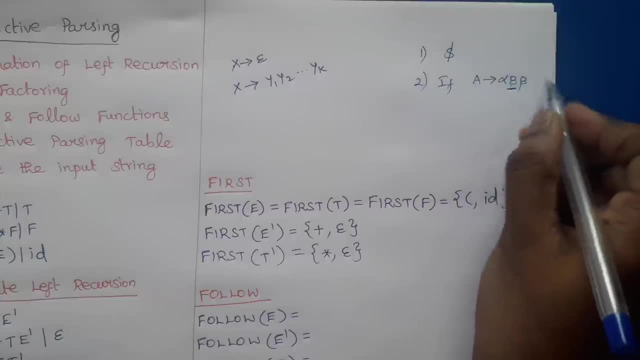 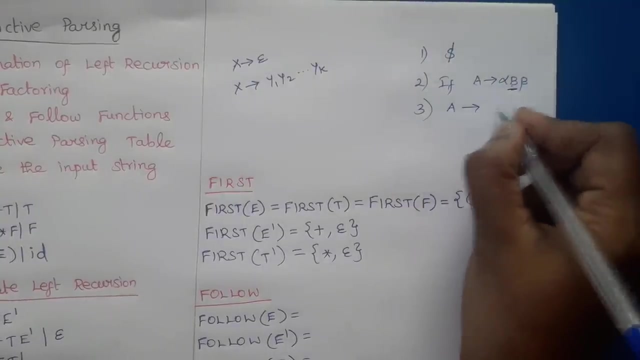 non-terminal. b is first of the string beta. Beta means it's a string First of the string beta except epsilon. So if all beta, all the symbols in beta deriving epsilon, then follow of b is a. So if a tends to alpha, b means if we want to find. follow of b means the b is followed by. 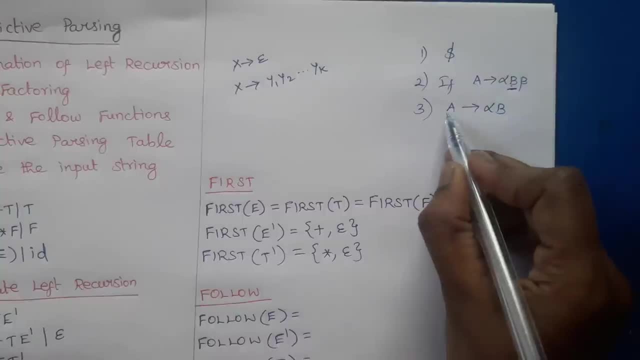 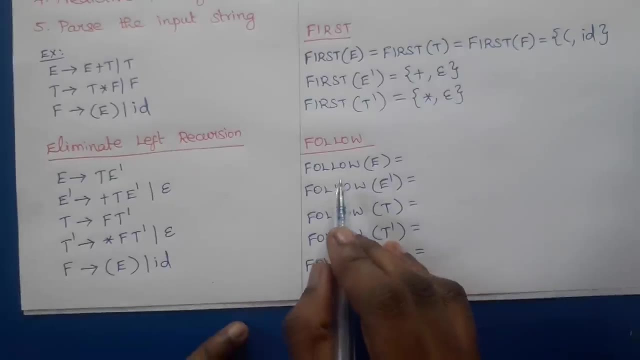 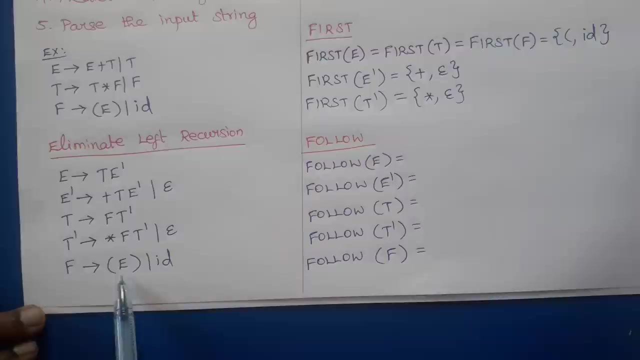 nothing here, no symbol. So follow of b is follow of a. So these are the rules for finding follow function. So first we need to find follow of e. So we have to check the right side of the productions. Here e appears in this production alone, So e is followed by right parenthesis. 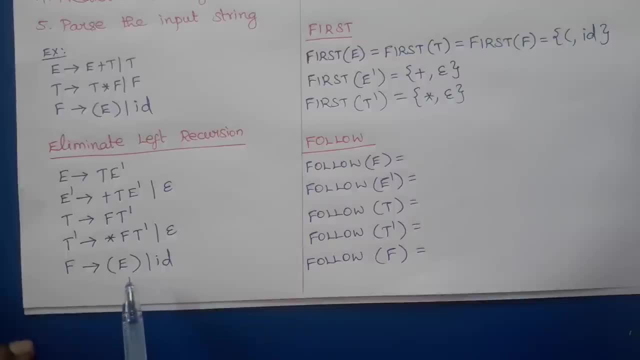 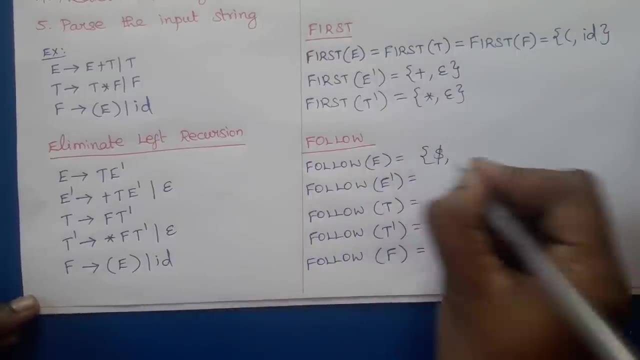 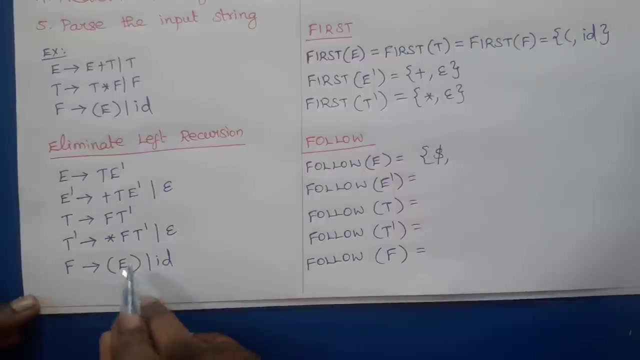 First of right parenthesis. First of right parenthesis is right parenthesis. And one more thing: since e is a start symbol of the grammar, we need to include dollar first. Then we have to find the check, the right hand side. Here e is followed by the terminal symbol. So first of 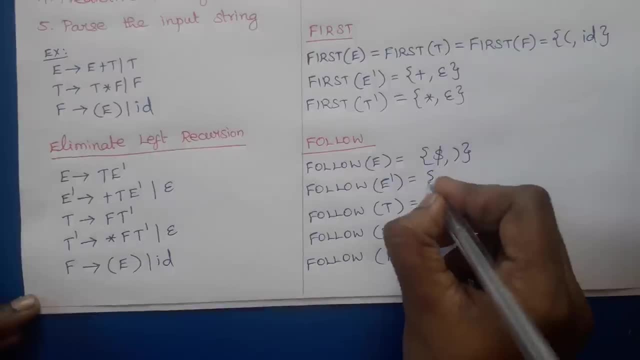 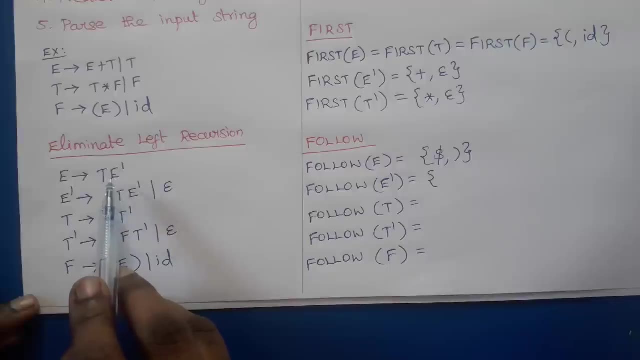 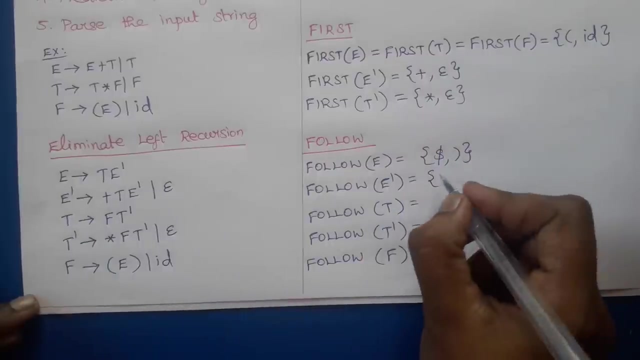 terminal is terminal. Then we need to find follow of e dash. E dash there are in two cases. First consider first case: follow of e dash. E dash is followed by the terminal symbol. So first of e is followed by nothing. So follow of e dash is follow of e. So what is follow of e Dollar and 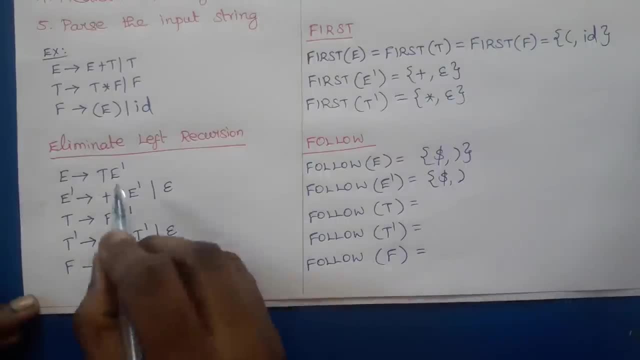 right parenthesis, Then in this case, follow of e dash is here also nothing. So follow of e dash is follow of e dash. It does not make any sense, So close this. Then we need to find follow of t. T is followed by e dash, Follow of t. So we need to find first of 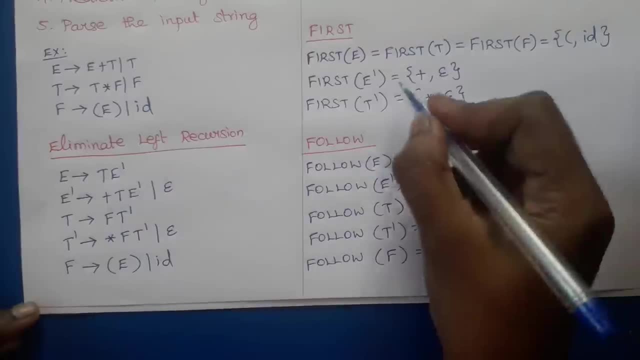 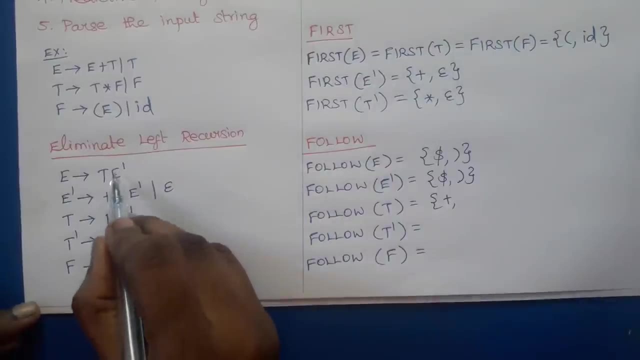 e dash First of e dash. So what is first of e dash Plus and epsilon? So e dash first of e dash is having epsilon here. So if we substitute epsilon here, then this e dash can be eliminated. So t is followed by nothing. So in this case we need to find follow of e also. So if you want to find 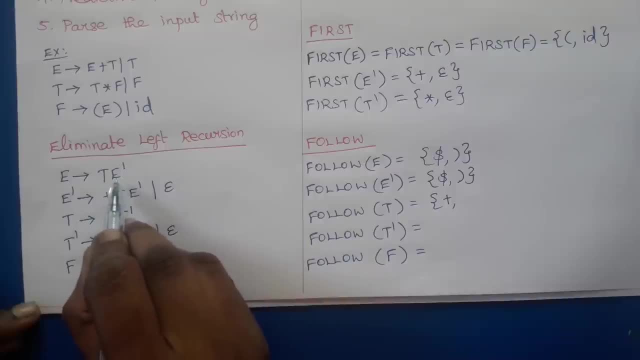 follow of t. First we need to substitute all symbols in first of e dash. So first of e dash is followed by e dash, So plus, except epsilon. So if epsilon is there we have to substitute epsilon, and if some other symbols are there we need to start finding first of that symbol. Here no, 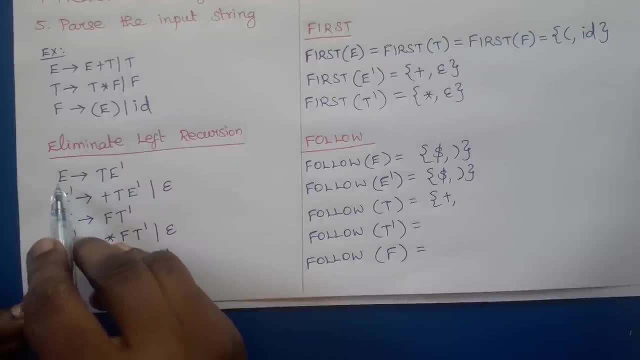 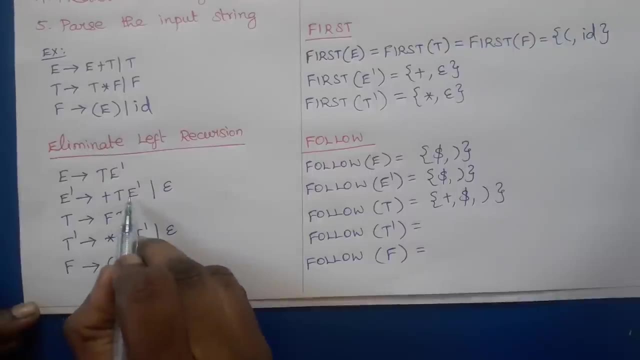 symbols, So we need to add follow of e also. So what is follow of e Dollar and right parenthesis. In this case also, t is followed by the same First of e dash, So first of e dash. now we have to include e dash, So we need to add follow of e. So what is follow of e Dollar and right parenthesis. 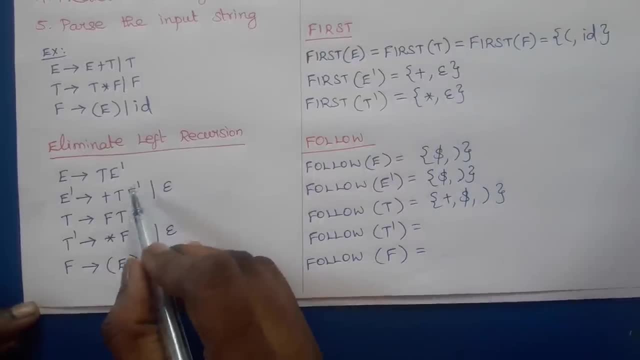 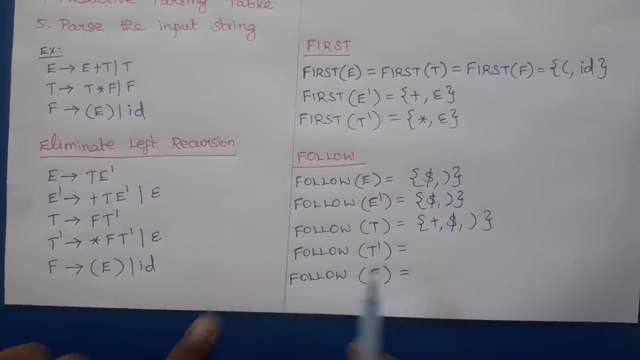 We include plus, Then if you substitute epsilon here we will find follow of e dash. So follow of e dash is also same thing. So follow of t is plus dollar and right parenthesis, Then follow of t dash. T dash appears in two cases, So here t dash is followed by no symbol, So follow of t dash. 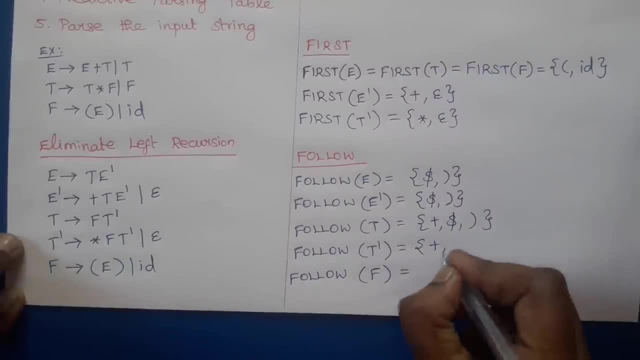 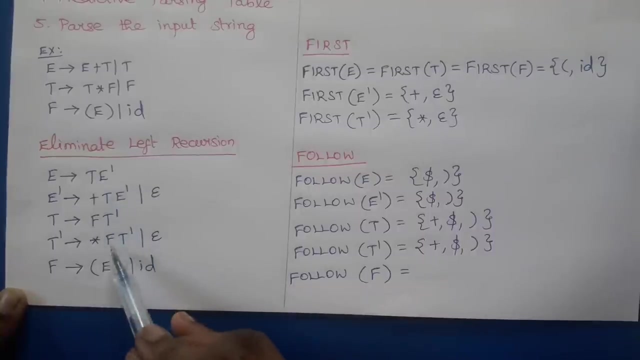 is follow of t, So plus dollar and right parenthesis. And in this case t dash is followed by no symbol. T dash is at the end of the prediction, So follow of t dash is follow of t dash. So no, it makes no sense. That's it Then. follow of f: F appears in these two cases, So follow of f is. 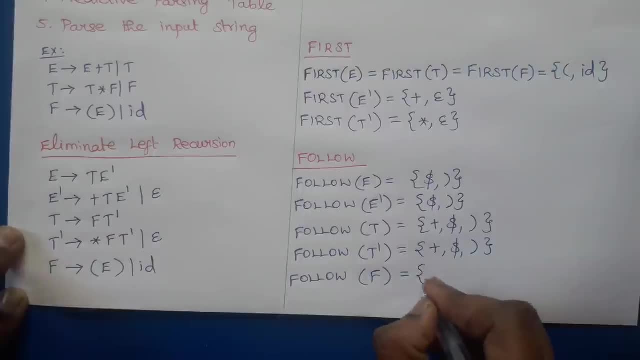 first of t dash. So what is first of t dash Star, And instead of epsilon in follow. epsilon should not be substituted. So if epsilon is that, then we can eliminate. we can substitute epsilon over here. So if you want to find follow of f. 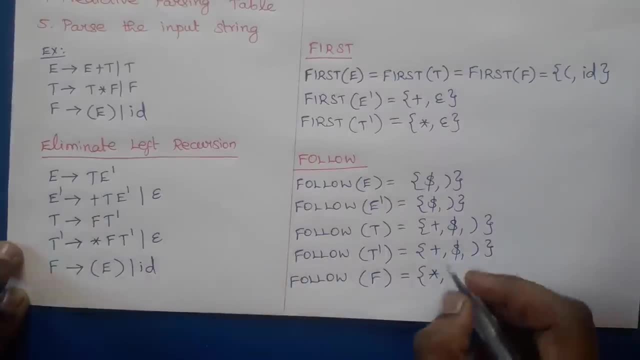 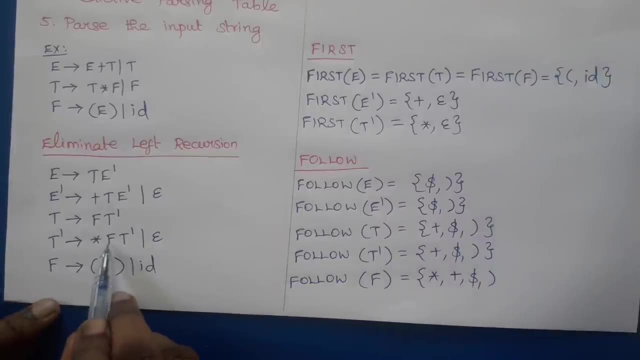 this will be eliminated. So follow of t should also be included. So plus dollar and close parenthesis, Then in this case also first of f. follow of f is first of t dash. First of t dash is star We have already included. Since epsilon is that we have to find follow of t dash also. 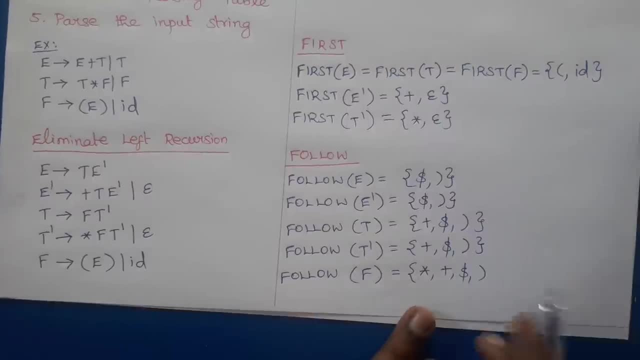 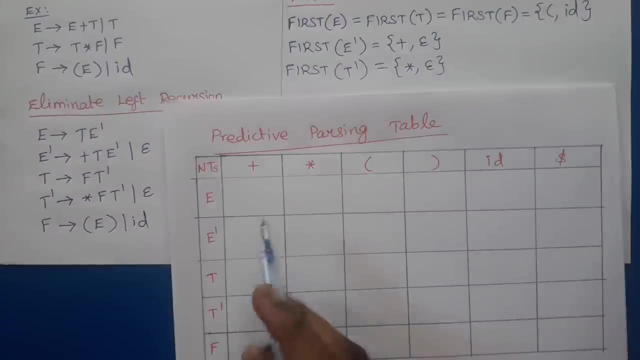 We have already substituted follow of t dash All the symbols in follow of t dash. So this is first and follow function for all the non-terminal symbols. Now the fourth step is finding predictive parsing table. So for finding predictive parsing table, rows are the non-terminals in the grammar. So e, e, dash, t, t, dash, f, These are the non-terminals. 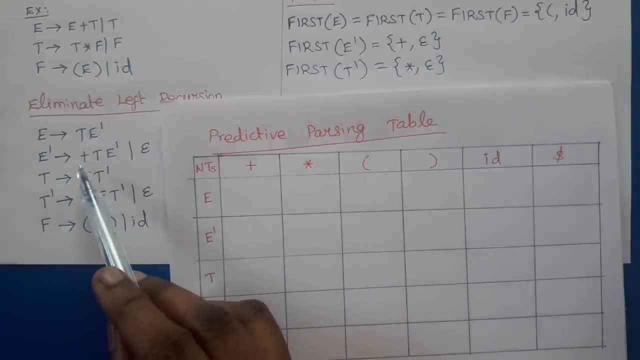 These are the non-terminals in the grammar. Then the terminal symbols are: plus star, left, parenthesis, right, parenthesis, id and dollar. So non-terminals are the rows, Terminal symbols are the columns in the grammar. Now we are going to substitute all the productions, So this is the 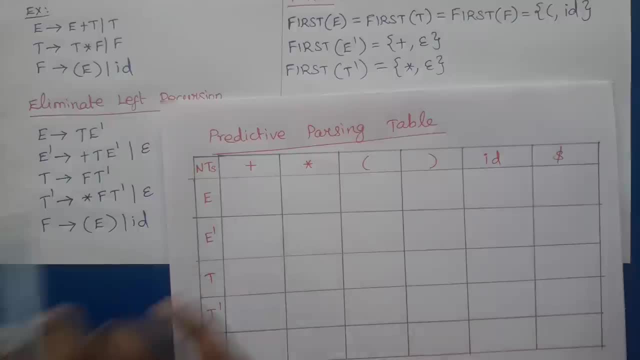 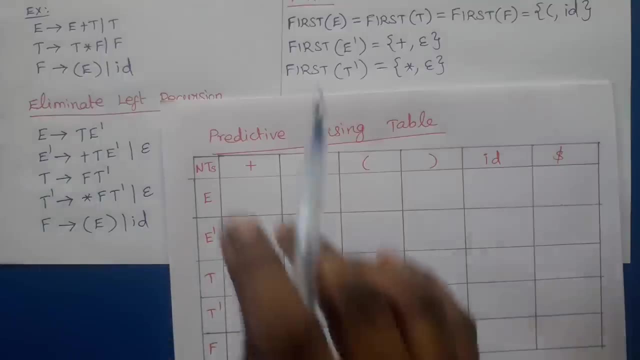 production. These are the productions we have got after eliminating elliptic recursion. So we need to substitute all these productions in the table. So the rule is that we have to substitute all the productions in the table. So the rule is that we have to substitute all the productions in the table. So 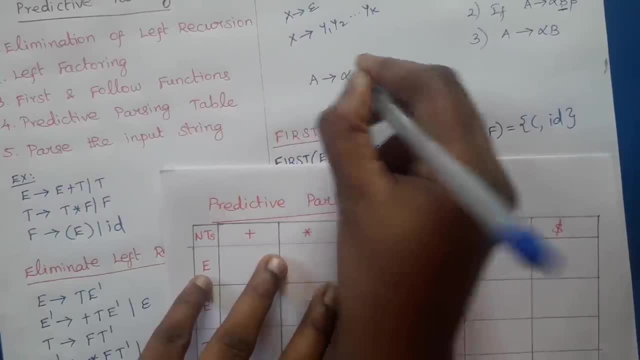 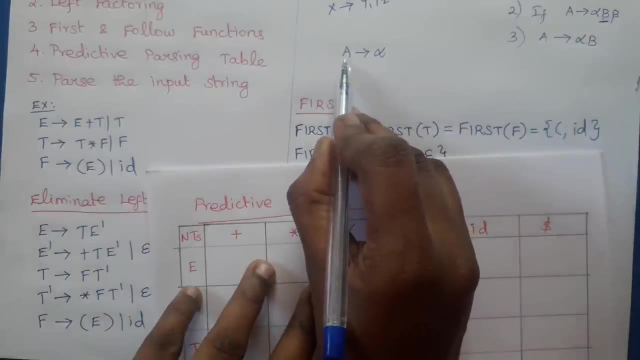 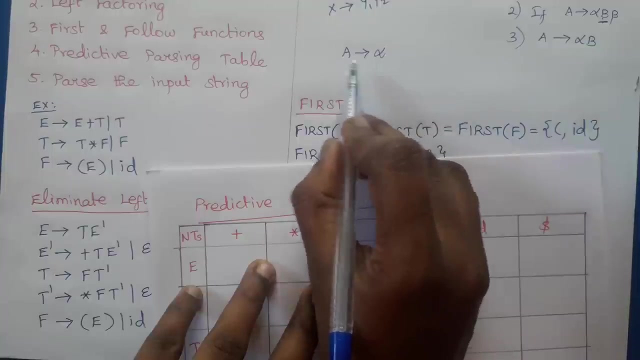 if a tends to alpha. If we are going to consider a tends to alpha, We should consider the row a, non-terminal a. Row for the non-terminal a should be considered and the columns are first of alpha. So in row a and first of alpha column we need to substitute this production a tends to alpha. 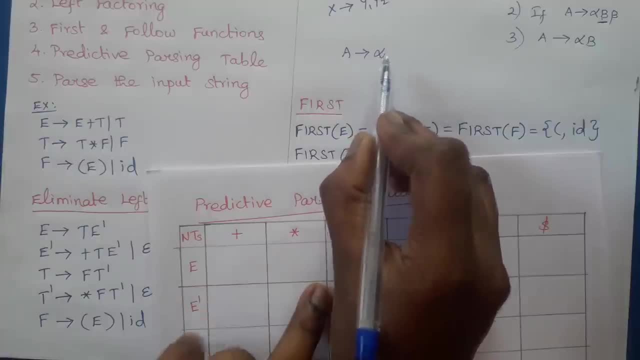 Suppose the first of alpha is having epsilon, Then we need to substitute. So this production in row a and columns Columns are the follow of the non-terminal symbol a. So these are the two productions we need to. These are the two rules we need to consider. 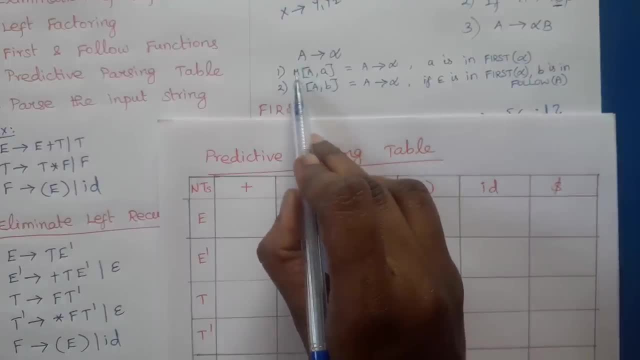 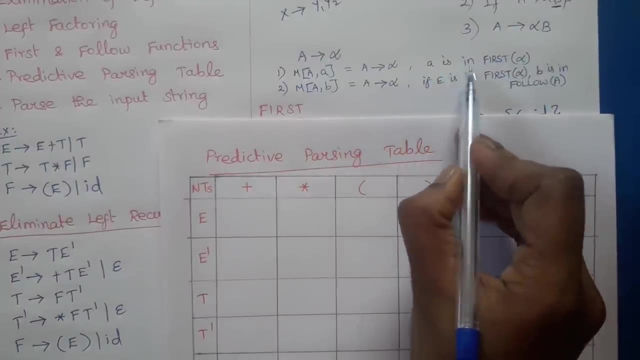 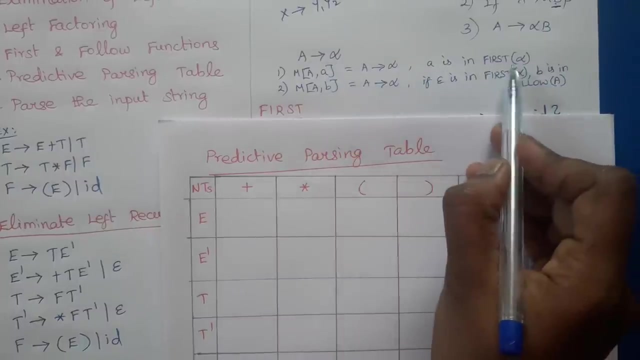 So m represents the table parsing table. Parsing table of the row a and column small letter a. Small letter a means it is in first of right hand side of the production. So follow of a. Sorry, first of all the symbols in right hand side of the production. So m of a comma. small letter a is 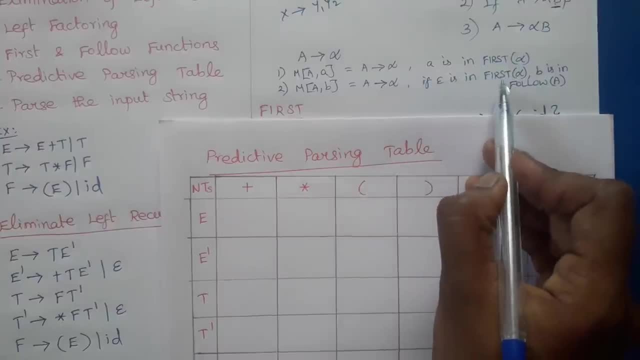 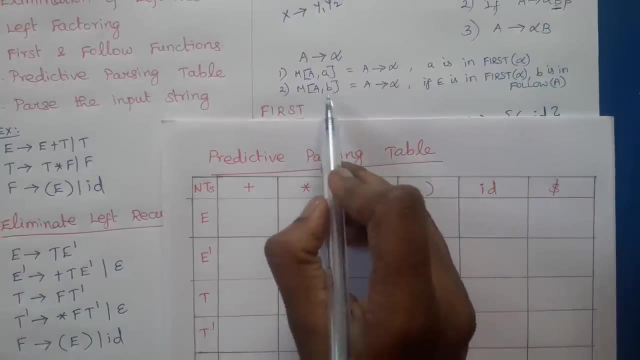 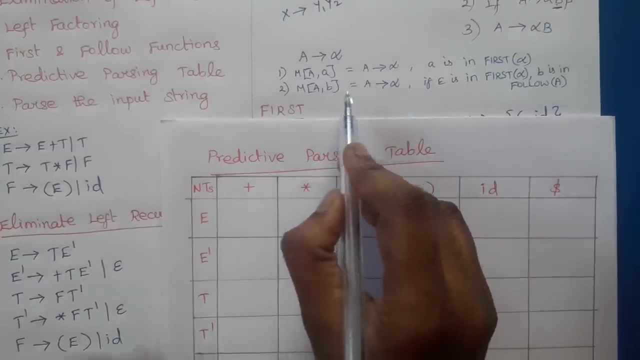 equal to a tends to alpha. If epsilon is in first of alpha, then we need to find follow of a. Suppose assume that b is a follow of a. So for all the symbols in follow of a we need to add this: production: a tends to alpha to m of a comma b. So these are the two rules. So now we are going to 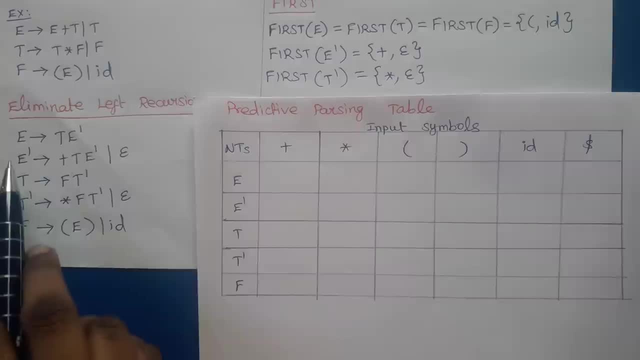 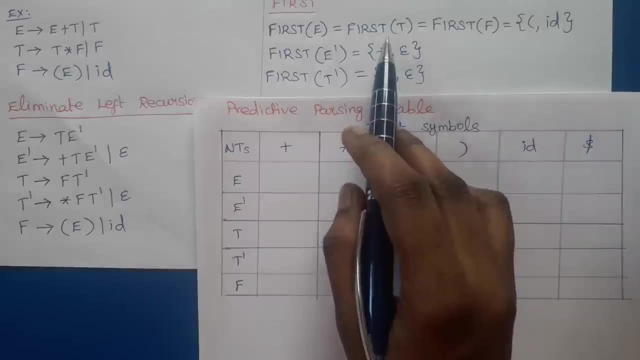 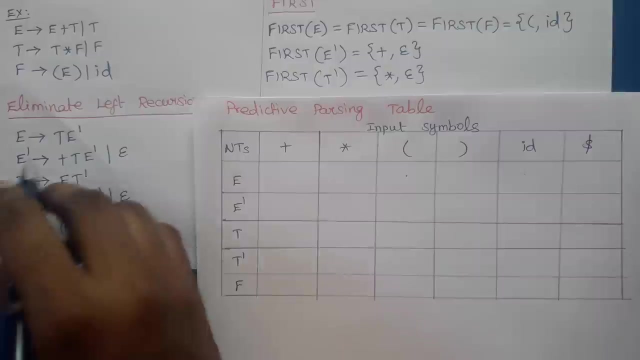 construct the predictive parsing table. Now the first production is e, tends to t, e dash. So first we need to find first of t. First of t is left parenthesis and id. So in row e and left parenthesis and id we need to write the production. 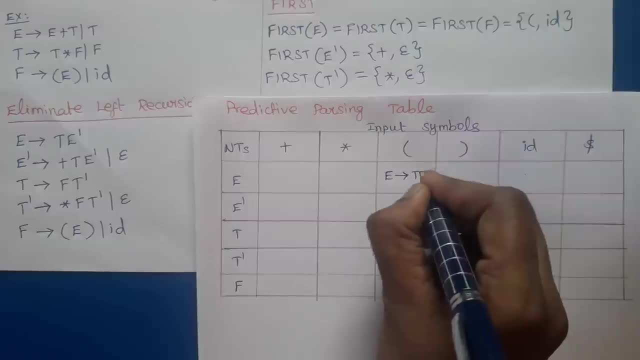 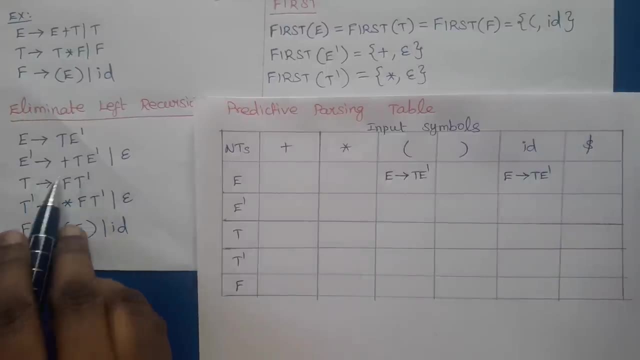 e gives t e dash. Then consider the second production. e dash tends to plus, t e dash First of the right hand side of the production. So first of plus t e dash. So first of plus t e dash, First of plus is plus. So in e dash and plus we need to write e dash tends to this production. 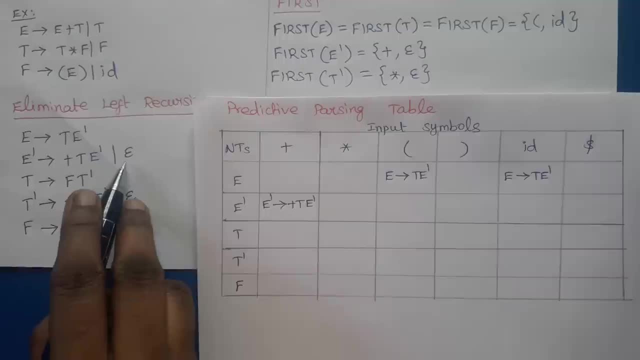 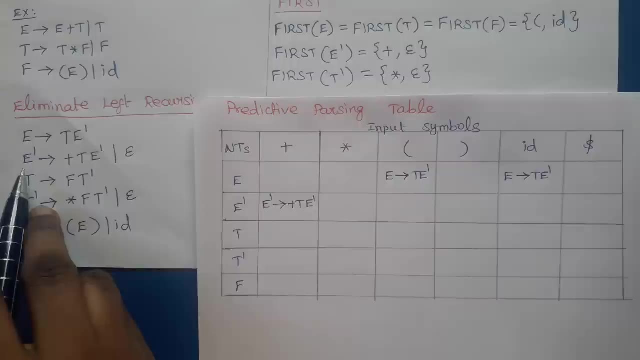 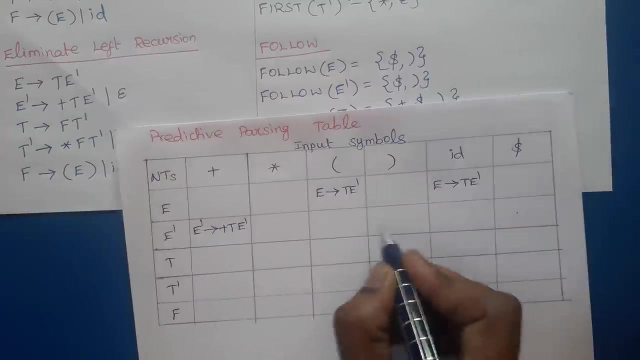 plus t e dash, Then e dash tends to epsilon. If epsilon is in right hand side we need to find the follow of e dash. So follow of e dash is dollar and right parenthesis. So in dollar and right parenthesis we need to write: e dash tends to epsilon, e dash tends to epsilon. 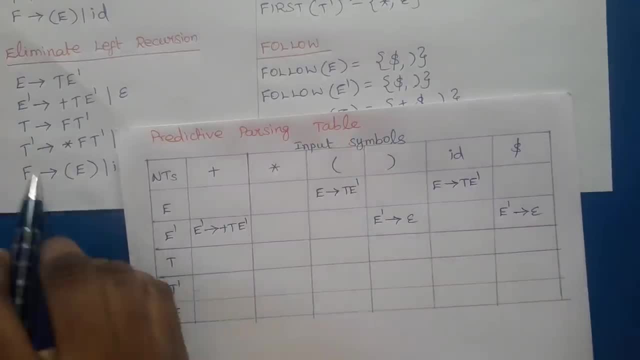 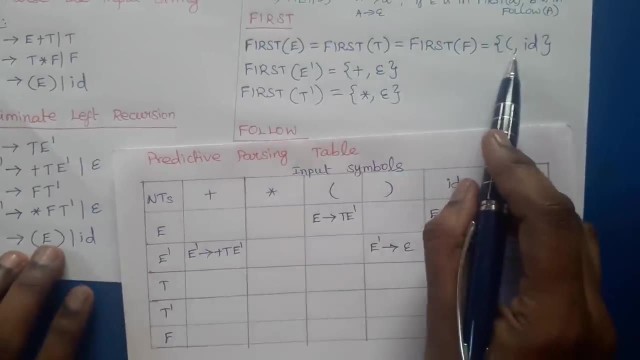 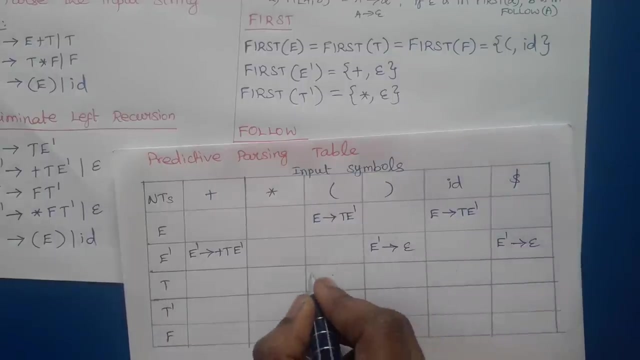 Should be written. Then t tends to f, t dash. So find first of f. First of f is left parenthesis and id. So in t and left parenthesis and t and id we need to substitute t tends to f, t dash. Then t dash tends to star, f, t dash. So first of star is star, So t dash and. 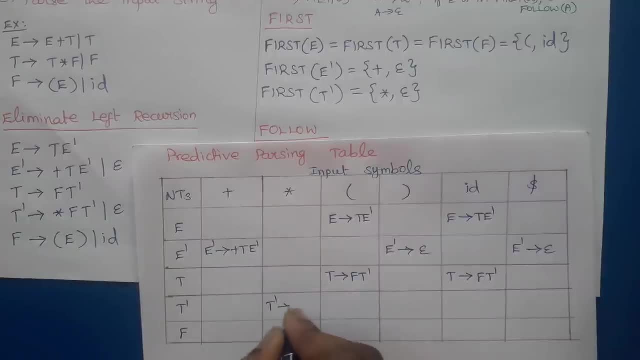 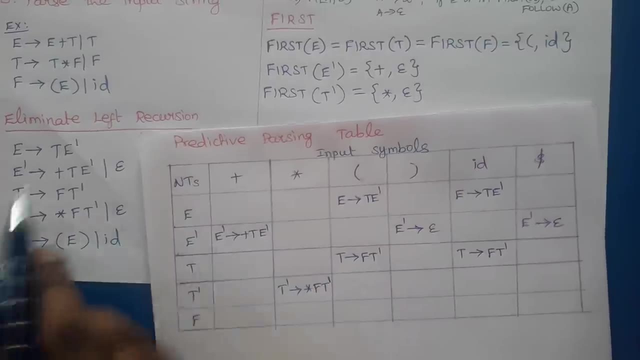 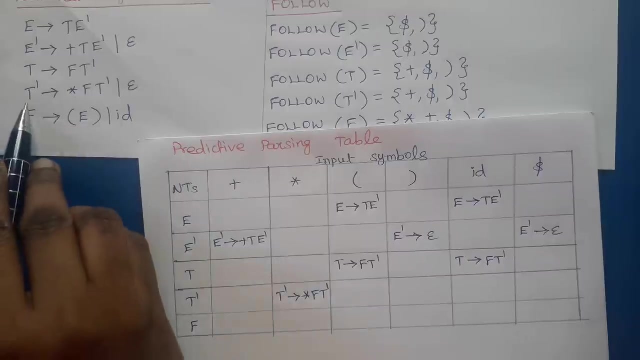 star. In t dash and star we have to substitute t dash tends to star f t dash, Then t dash tends to epsilon. So we need to find follow of t dash. Follow of t dash is plus dollar and right parenthesis. So in t dash non-terminal t dash and follow of t dash plus dollar and right. 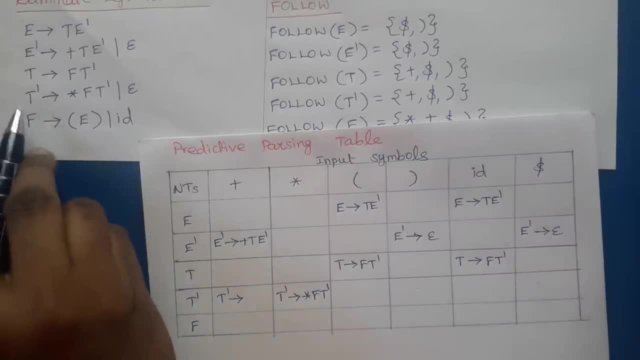 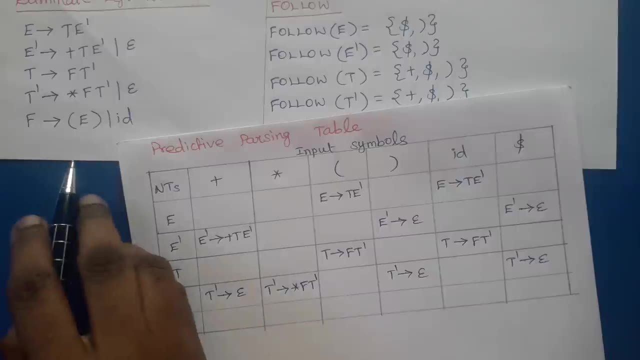 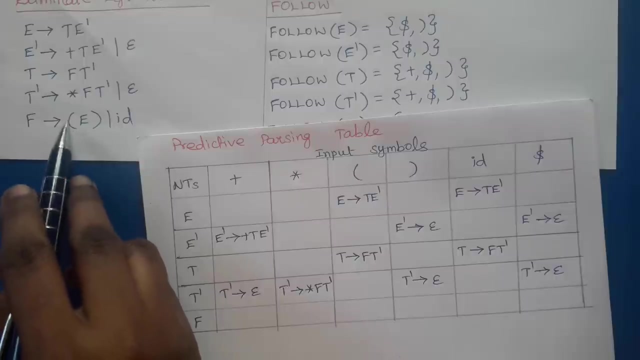 parenthesis In these three places we need to substitute the production. t dash tends to epsilon, Then consider this production. So to substitute this one we need to find first of left parenthesis, First of terminal is terminal, So f and left parenthesis in this column, f and left parenthesis. 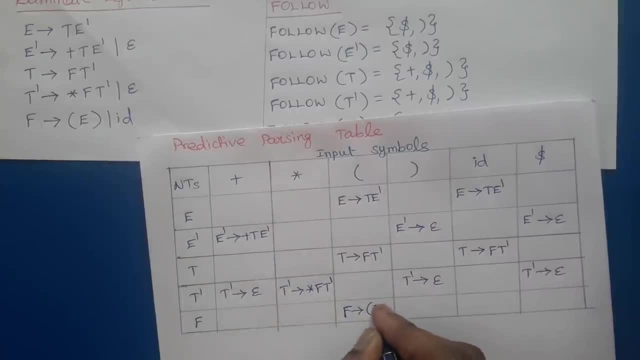 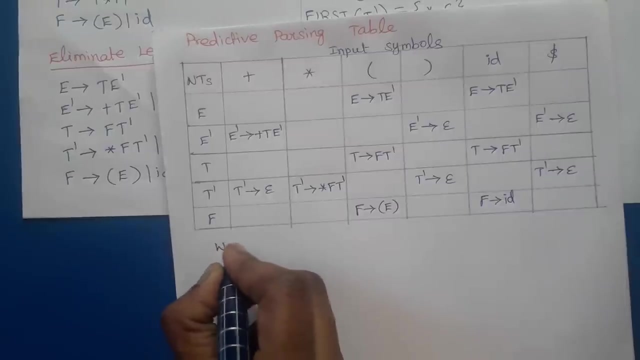 we need to substitute f tends to open parenthesis, e close parenthesis. Then f tends to id. First of id is id, So in f and id we need to substitute f tends to id. Now we need to parse the input string- w is equal to id, star id plus id by using this: 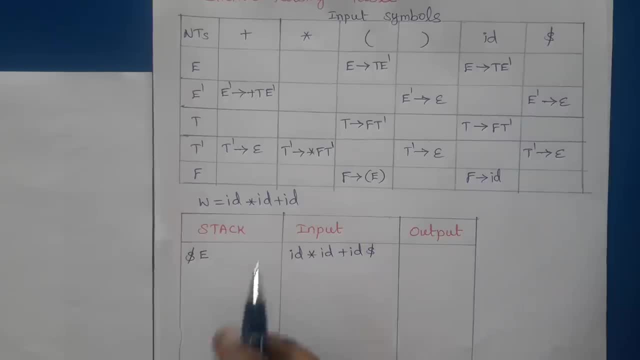 predictive parsing table. So to parse the input string we have to consider stack, input and output. Predictive parsing table uses stack as a memory unit, So the initial configuration of the stack is dollar and e Dollar represents bottom of the stack. and then we need to load. 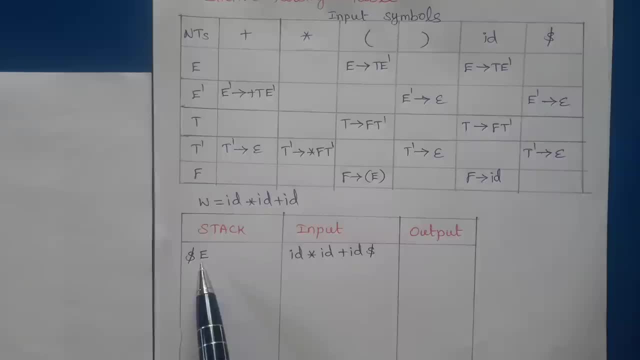 the start symbol of the graph. So we need to load the start symbol of the graph. So we need to load the grammar onto the stack. So now the top of the stack is start symbol of the grammar e. Then in input buffer we need to store the string to be parsed So id, star, id plus id. This w w means. 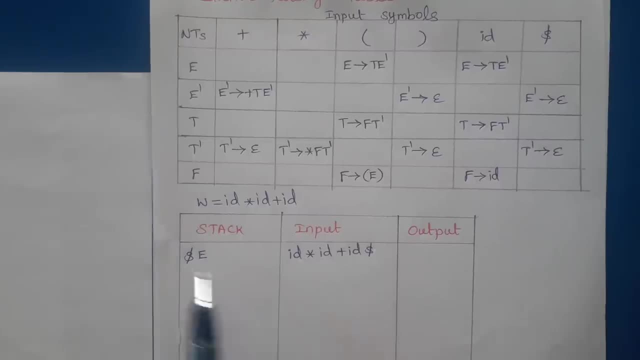 input string should be followed by dollar, W followed by dollar. So the initial configuration of the stack is dollar. start symbol of the grammar Input buffer is w and dollar. Then we have to remember two things. If the non-terminal is on top of the stack and input pointer points to id any input symbol, then 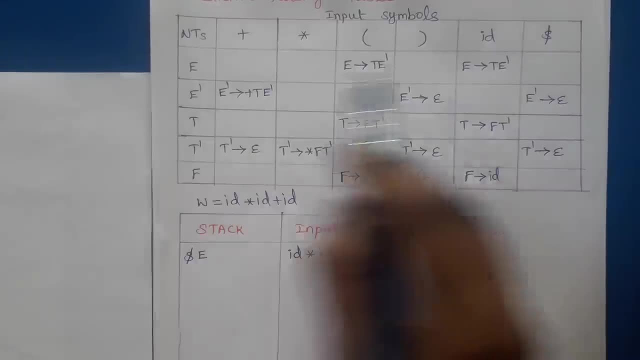 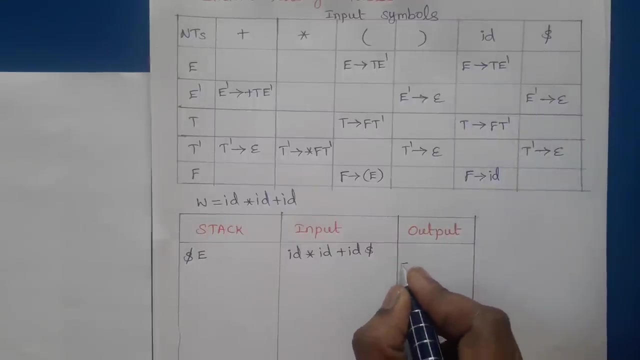 we need to refer the predictive parsing table e and id. So e and id means we will get some production, So that production should be written in the output. Then left side of the production, that is e, should be on top of the stack. So that should be replaced by the symbols on the right. 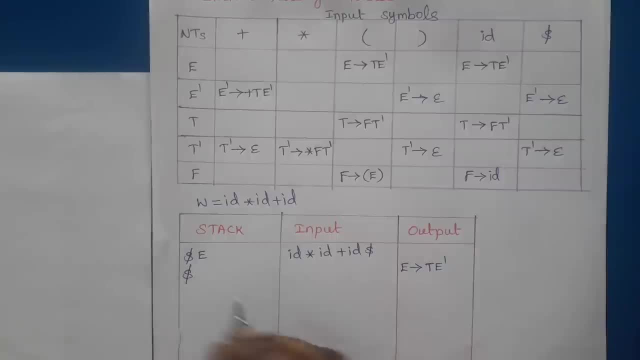 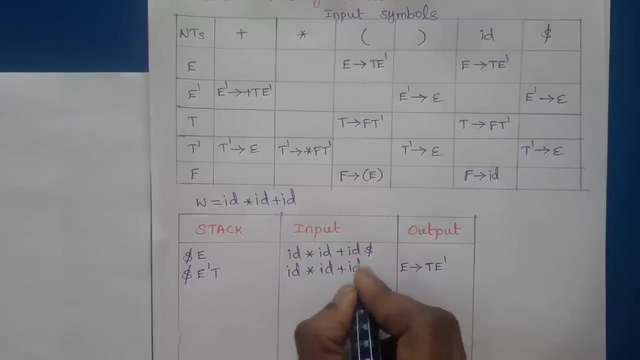 hand side of the production In reverse order. So dollar e is popped and we need to push e dash nt. So t must be on top of the stack and no change in input buffer. So if a non-terminal is on top of the stack and the 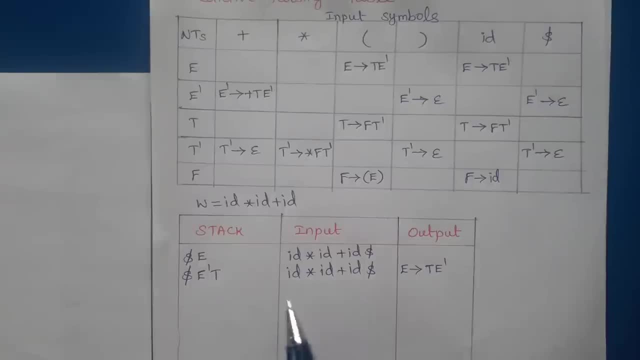 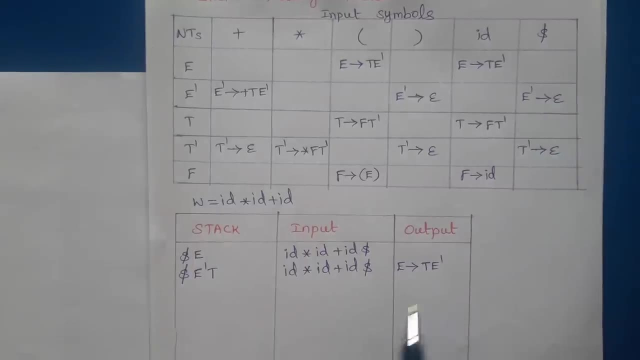 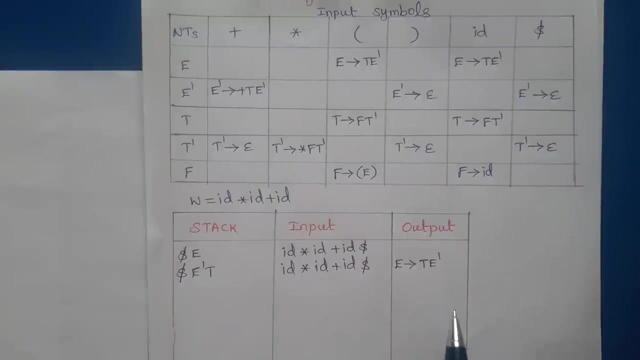 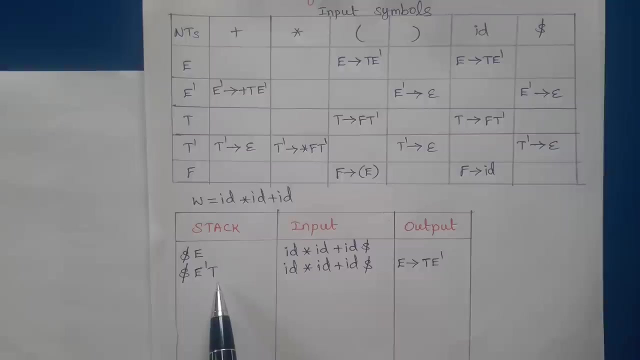 current input symbol is any terminal symbol. we need to refer the parsing table- predictive parsing table- and output the production in the output column. Sometimes a terminal symbol may be on top of the stack, So that should be. if the terminal symbol is on top of the stack, that must be matched with the current input symbol. And if they matches then we can. we can pop the terminal symbol on top of the stack and foundation For an Mass Gllo platform filter we need to have ages. This is where we have cleaned all the inputs of ohm size sheets And for the e fixation error we need to reply the setter symbols on top of the stack. this is our program for this example. This is theắn terminal code in this example. Now there are a few evidences. E fixations are available in url that we store, Or maybe you have a cursor where we should put the add strings. 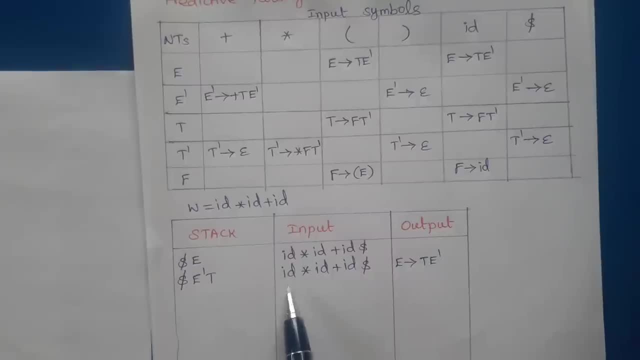 We need to enter theил icon By ashalten edges and press entonces NFL index. or here we put the index letter number. here for this interval, remove the input symbol from the input buffer, that is, we have to advance the input pointer to the next input symbol. These are all the two cases we need to remember Non-terminal means we need. 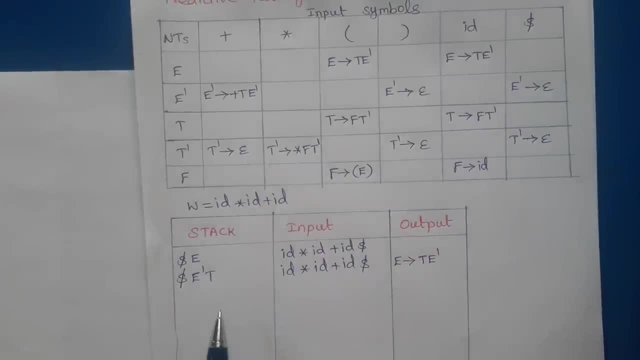 to refer the predictive parsing table Terminal means match the symbol with the input buffer and pop it. So finally we need to get dollar and dollar Dollar on top of the stack. the meaning is stack is empty and input buffer should also contain dollar. Then only we can say that the 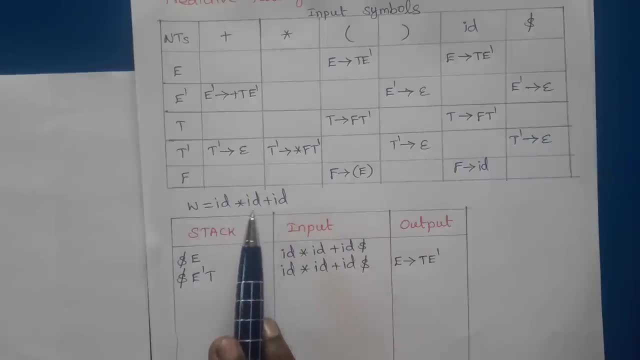 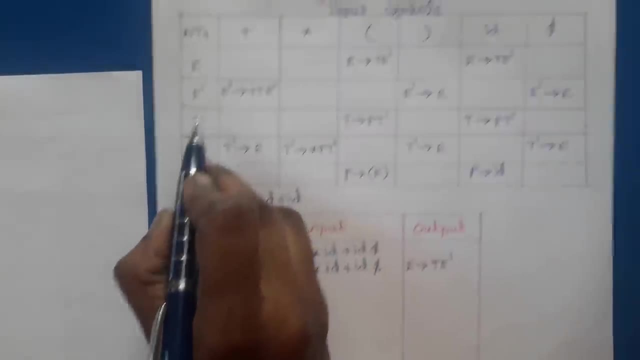 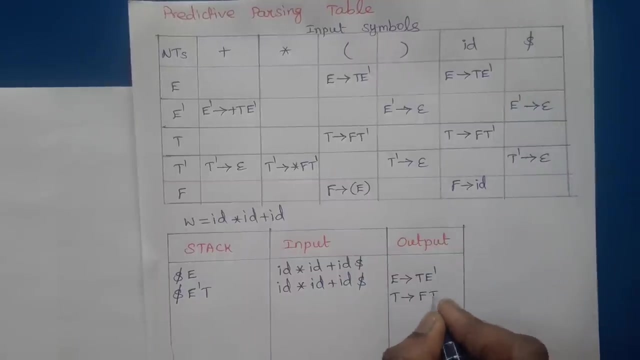 input string is accepted. We have successfully derived the input string from the start symbol of the grammar, So we will do this. So now t and id, So t and id. Yes, t tends to f t dash, So write t tends to f t dash here. So replace t means pop t and push t dash and f, in reverse order. 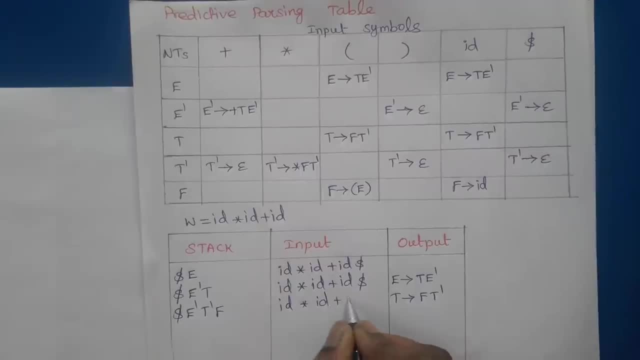 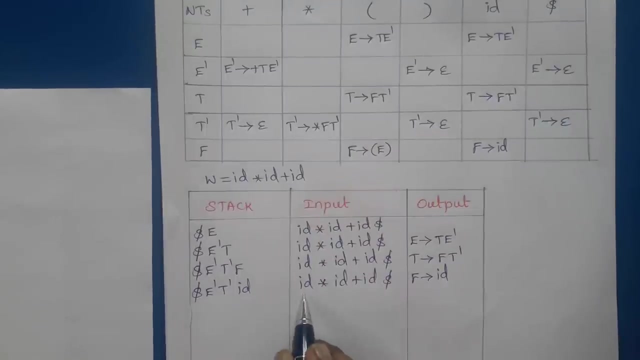 id, star, id plus id. No change in input: Now f and id. So f and id is f tends to id, So pop f and push id. Now the top of the stack is terminal symbol, So this is matched with the current input symbol, id, So we can remove both. 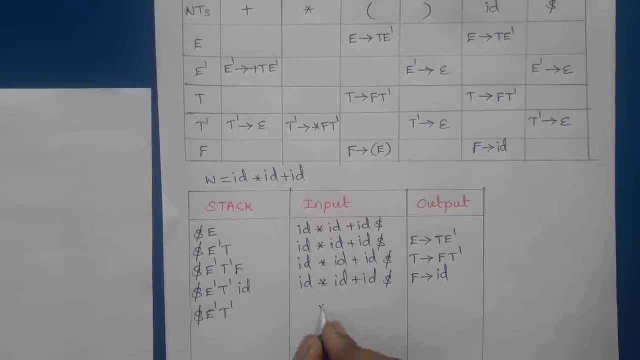 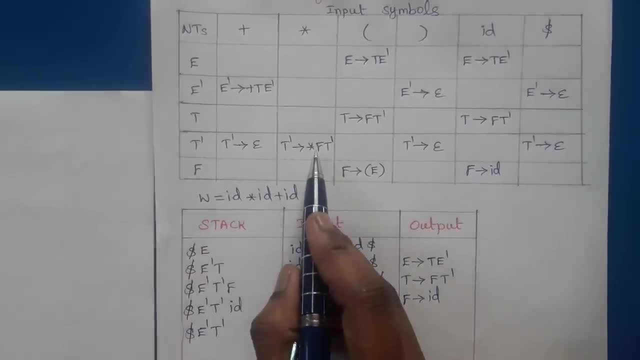 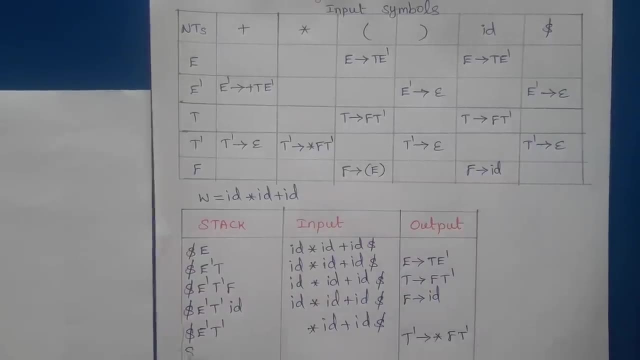 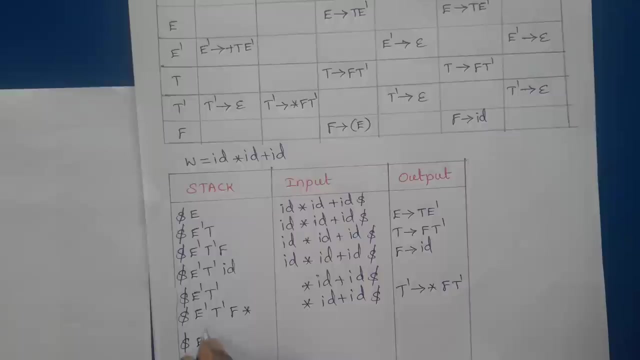 News: star and star, So t dash and star Means t dash tends to star f t dash. That should be written in the output. and remove t dash from the stack and push t dash f star. Now star and star, So remove it Here also remove. 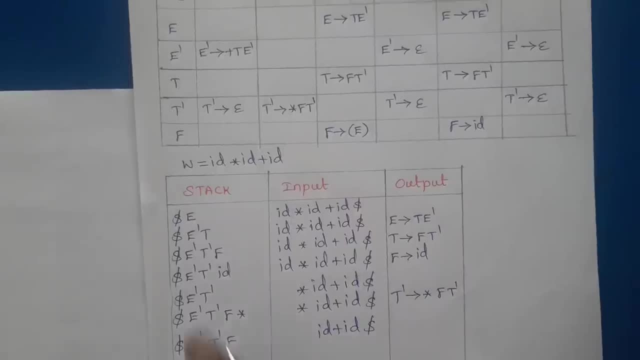 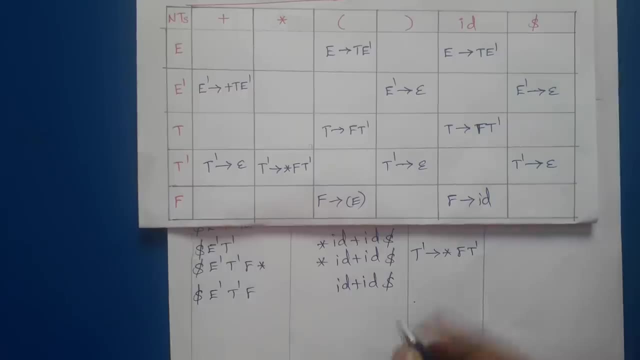 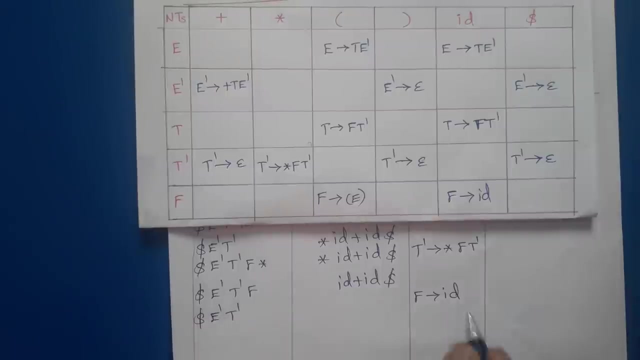 now f and id. so f and id is f tends to id. so that should be written in the so f tends to id. so pop f from the stack and push id now id and id. so remove both. now t-das and plus. so refer the table t-das and pluses. t-das tends to epsilon. 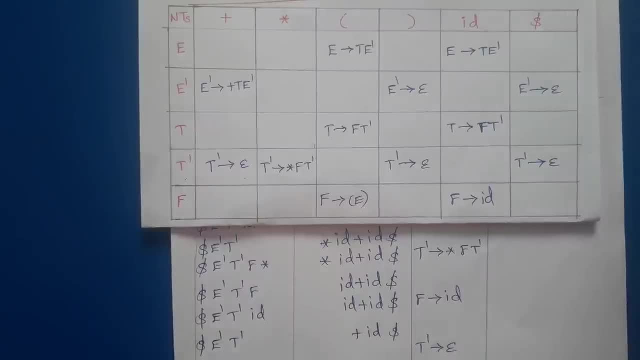 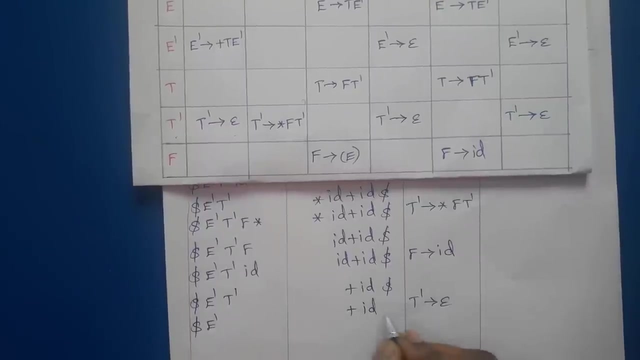 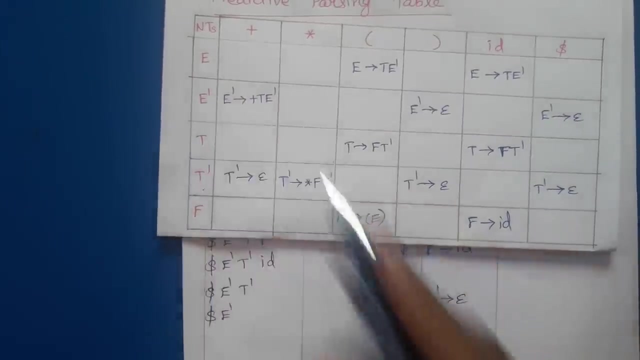 so t-das tends to epsilon, pop t-das and push epsilon. epsilon is pushed means no need to write that, just write e-das alone. then plus t plus id dollar here, then now e-das and plus. so e-das and pluses, e-das and pluses. 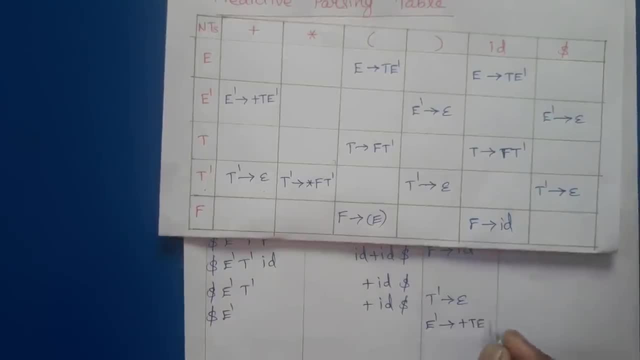 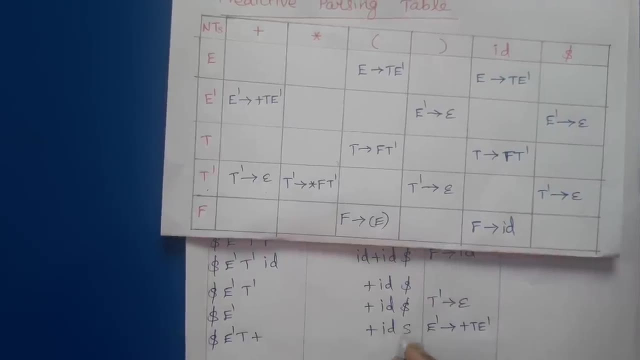 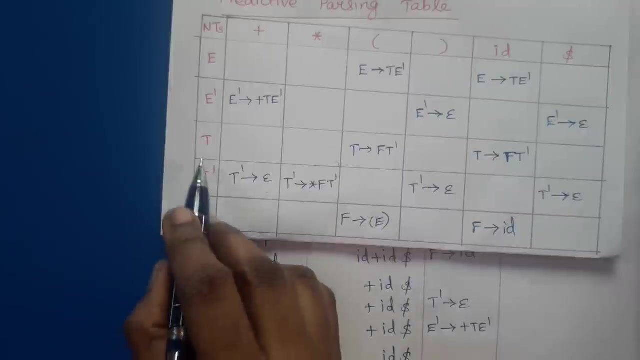 so e-das and pluses E dash tends to plus T E dash. So pop E dash and push E dash. T plus Here, plus ID dollar Now plus and plus. So remove both. Now T and ID. T and ID is T tends to F T dash. 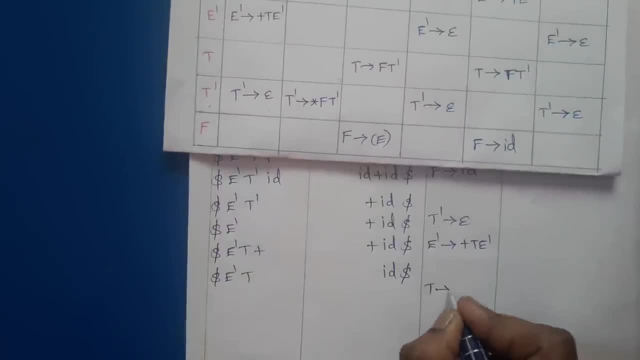 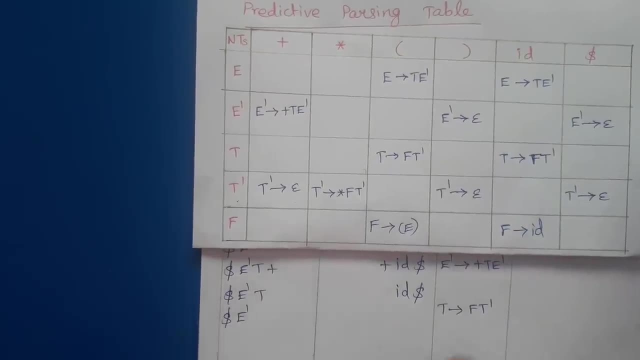 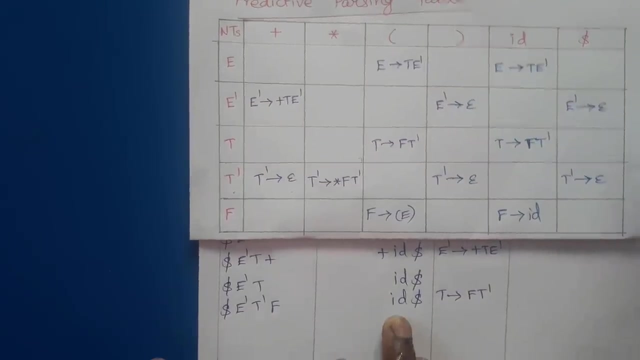 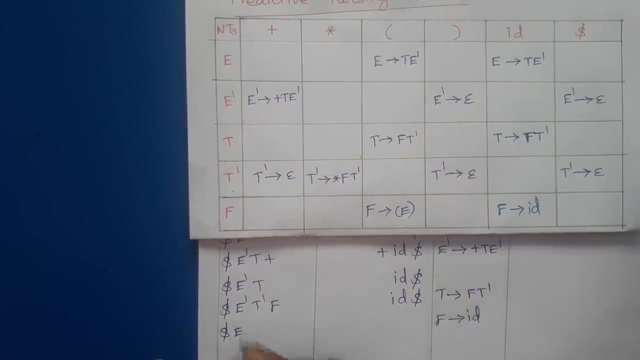 So T tends to F. T dash Plus means pop T from the stack and push T, dash F, Now F and ID. So F and ID is F tends to ID. So write F tends to ID first, Then pop F and push ID. 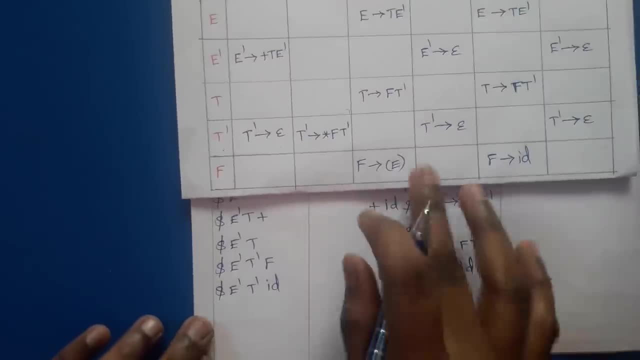 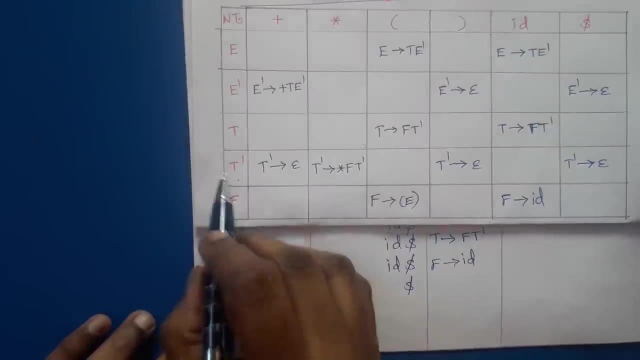 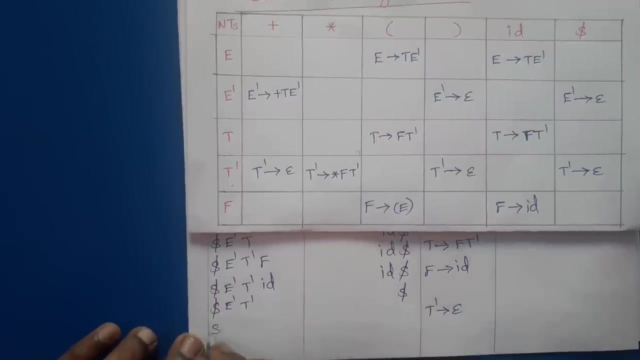 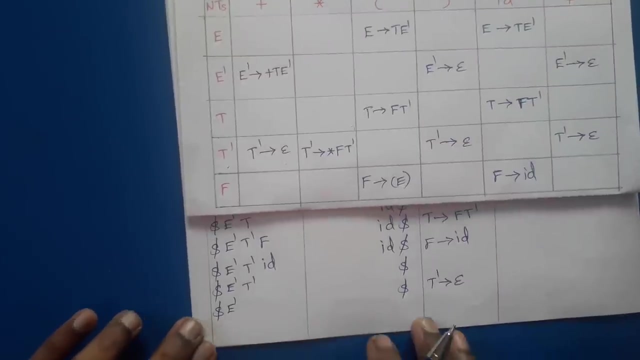 Now ID and ID can be removed. So T dash and dollar. T dash and dollar is T dash tends to epsilon, So T dash can be popped and push. epsilon Means no need to write anything, Then E dash tends to dollar. 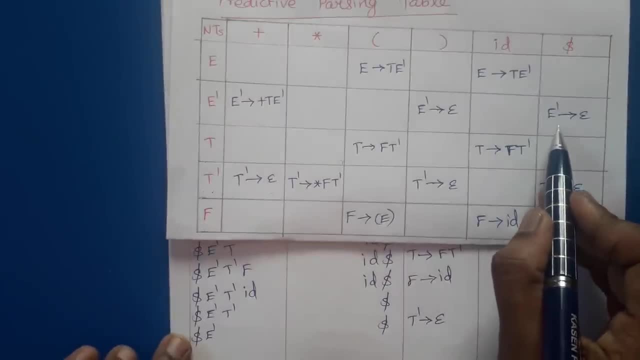 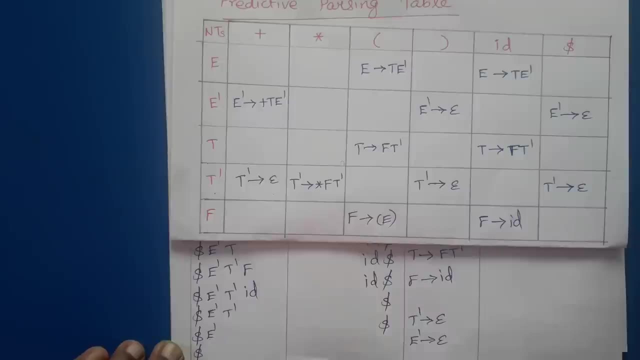 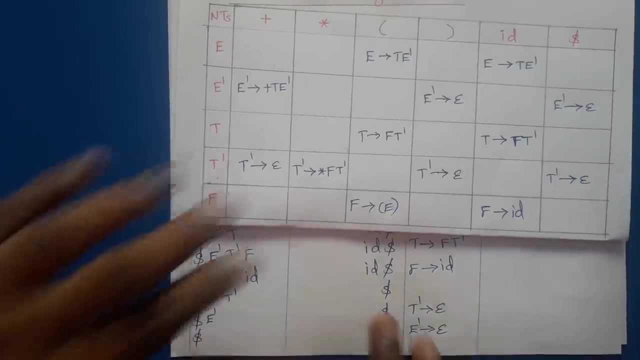 E dash tends to dollar, is E dash comma. dollar is E dash tends to epsilon. So E dash, E dash can be replaced by epsilon. So now we have got dollar and dollar Stack is empty. Input buffer is also empty. So these are the output set of output productions we have got. 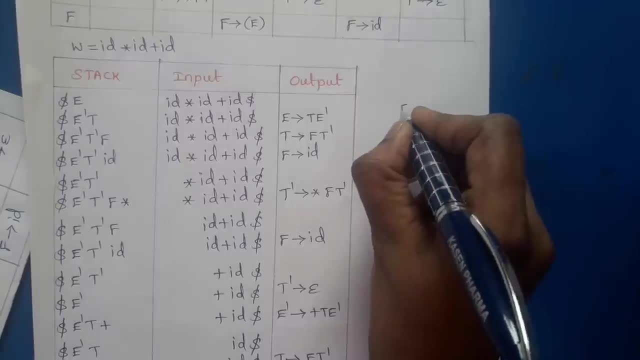 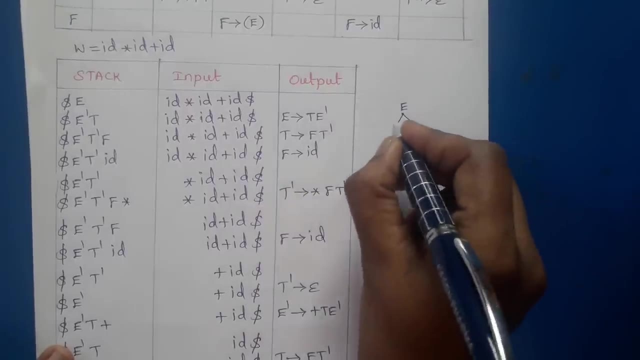 So if we start constructing the parse tree from the start symbol of the grammar E First, we have got the output E tends to T E dash. So E has the two children, T E dash. The T can be expanded by using the second production. 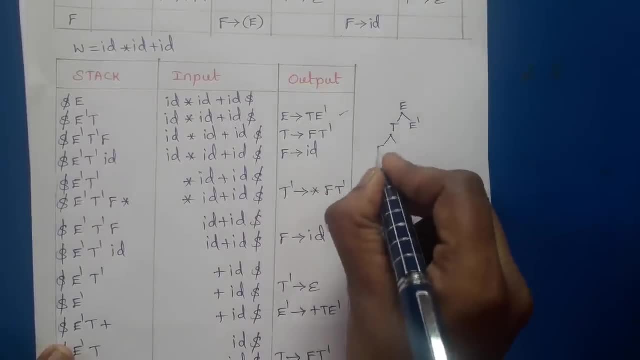 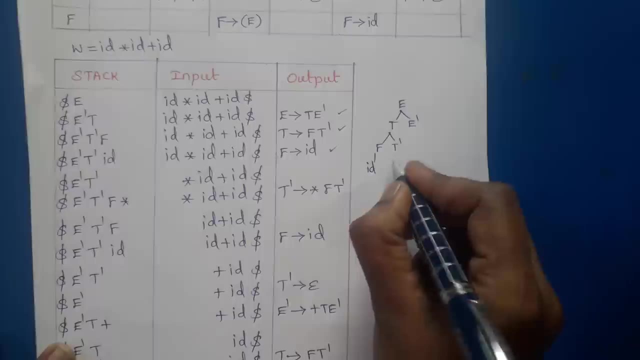 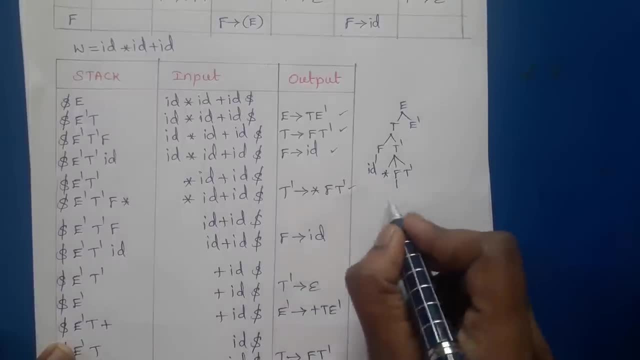 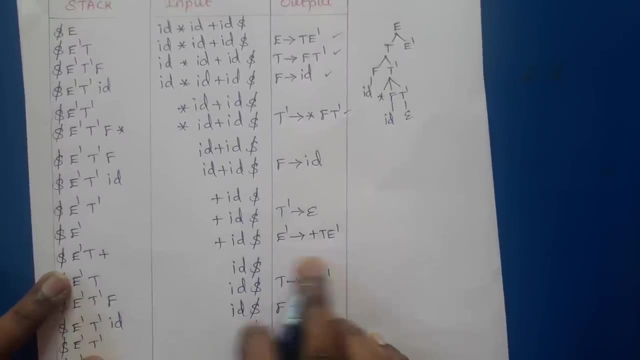 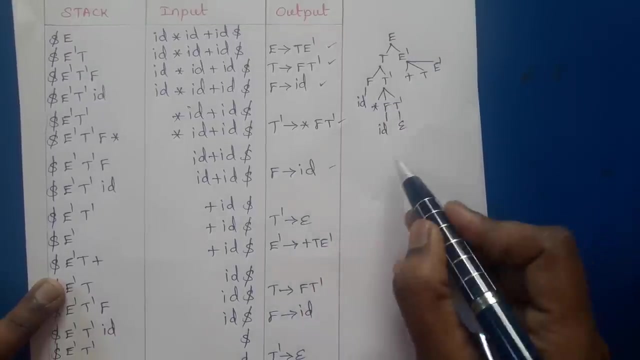 Star F T dash, Then F is replaced by ID, Then T dash tends to epsilon, Then E dash tends to plus T E dash. F tends to ID over T dash tends to epsilon, Then E dash is expanded by using plus T E dash. 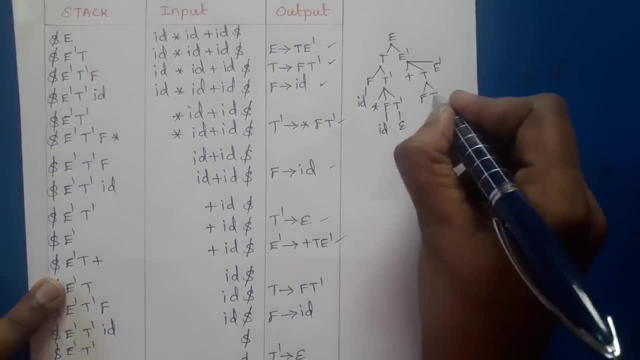 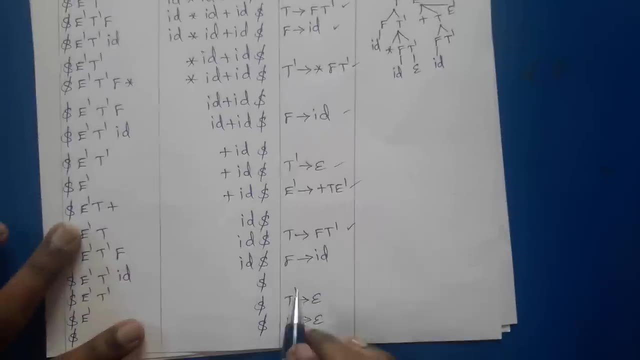 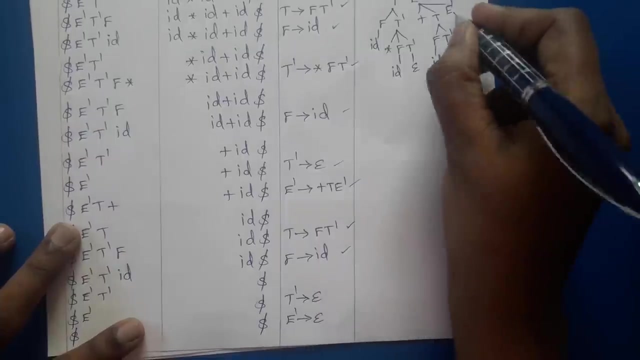 Now T tends to F T dash, T tends to F T dash. This is also over. Then F is replaced by ID. Then this T dash is expanded by using epsilon. Then E dash is replaced by epsilon. Now, if you concatenate, 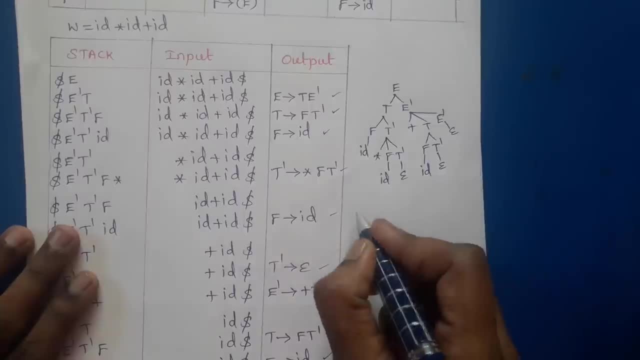 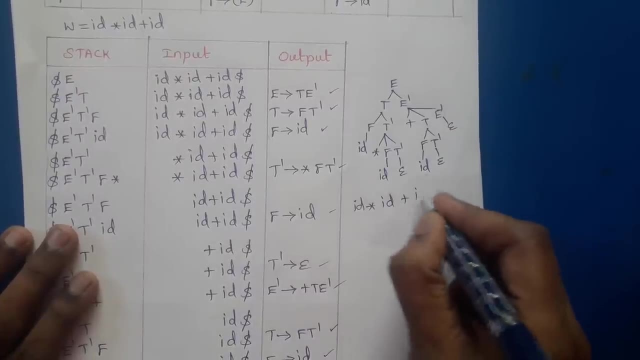 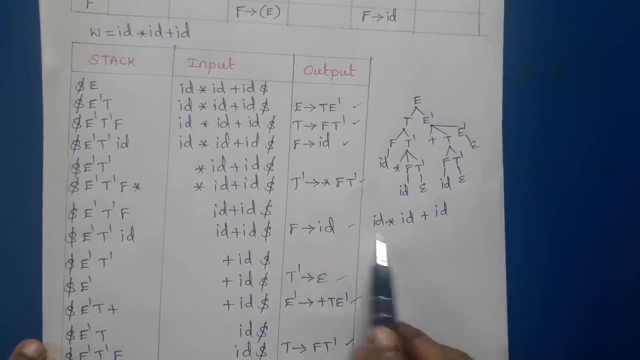 If you concatenate the leaves, the symbols on the leaf from the left end, you will get ID star ID plus ID. We can remove the epsilon because it's an identity element during concatenation, So we have derived the input string ID star ID plus ID. 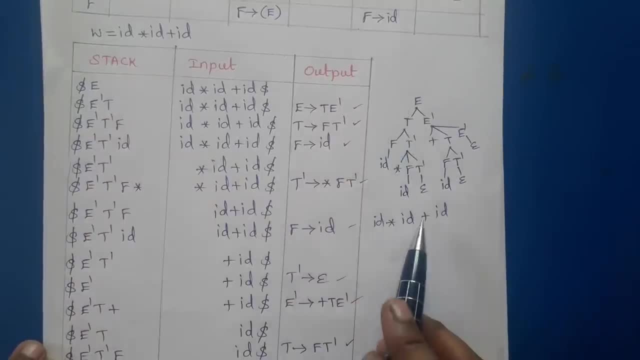 This input string is derived from the star symbol of the grammar successfully, So we have parsed the input string using predictive parsing table. Thank you, Thank you.